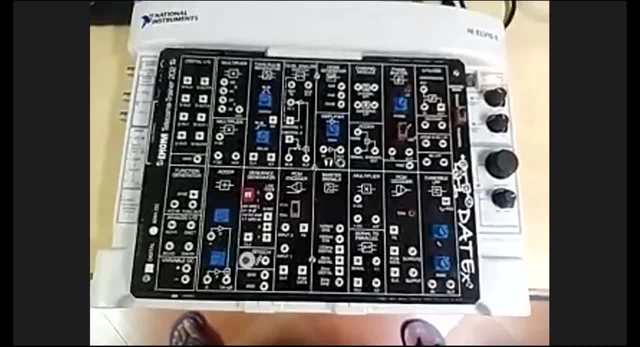 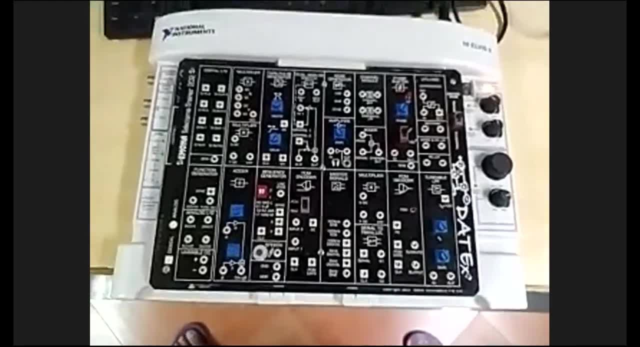 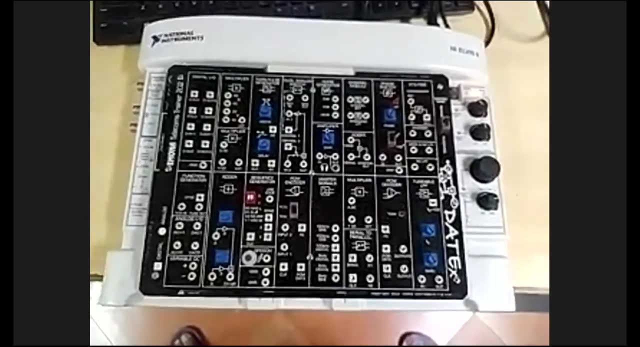 the background of the frequency phase shift keying. Frequency phase shift keying or the frequency shift keying, sorry- which in terms called FSK, is a frequency modulation scheme in which digital information is transmitted through discrete frequency changes of a carrier wave. For instance, if you have got a carrier wave and that carrier wave has got a continuous 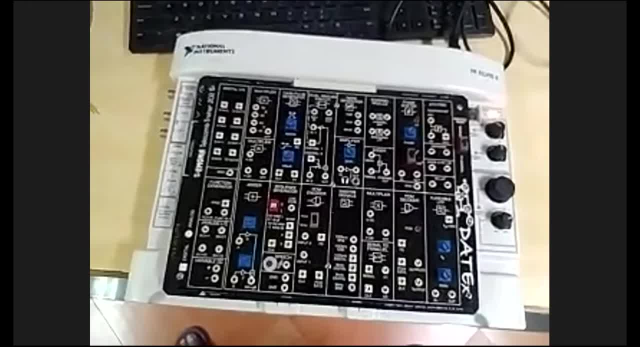 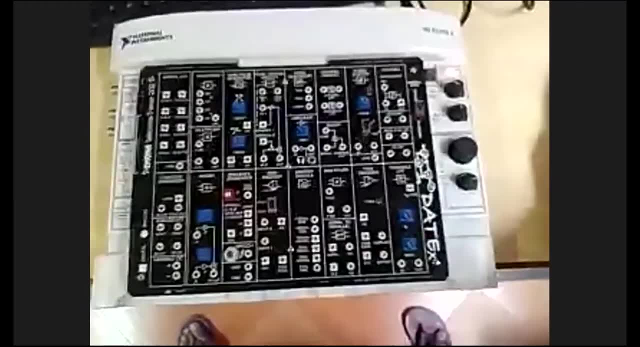 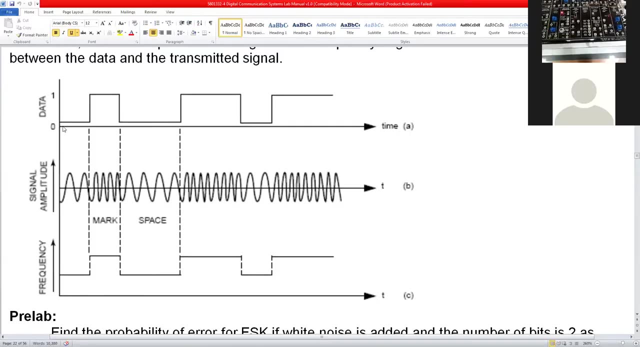 frequency, then this: that particular continuous frequency will be changed as per the transmitted or the baseband signal. That is the main theme of the frequency phase shift keying, For instance. you can see that we have got data over here. The data has got certain pulses with respect to the time, which means the data represents. 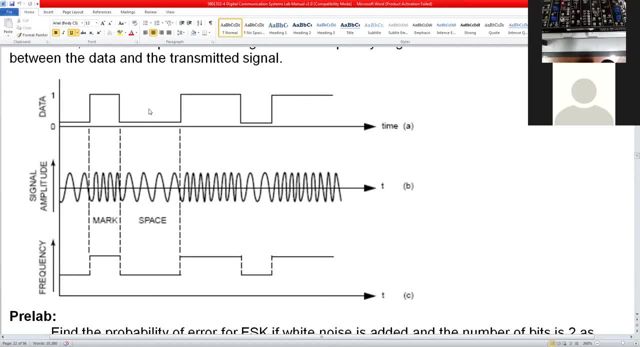 highs and lows. This can be represented by binary one And this can be represented by the binary zero. the low pulse or the pulse which has got no energy associated with it or the zero volt associated with it, can be termed as zero volts. 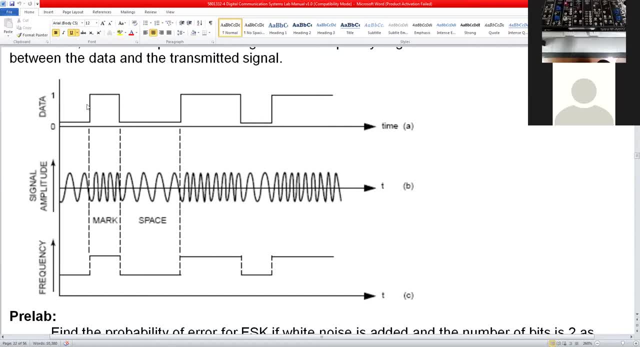 the zero, in terms of binary, and the pulse, which represents the maximum voltage of the system. for instance, that can be 5 volts or 10 volts and generally speaking we affects 5 volts with that particular system, the 5 volt system, the high voltage that can be shown in that particular. 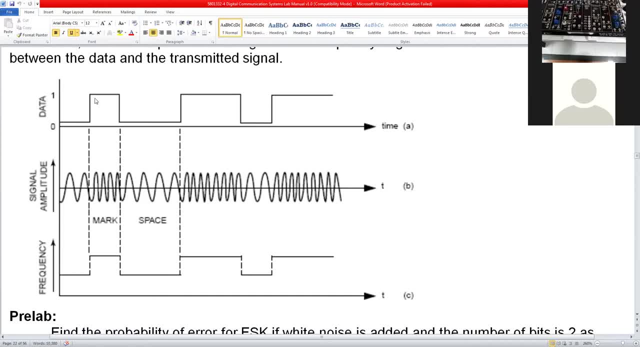 pulse we can show. we can take that as a binary one. so we have got one over here, then zeros, two zeros as per the time, and twos, two ones, then zero. so you can see that we have got a data with variables, ones and zeros, that that I can be modulated by a continuous wave since previously. 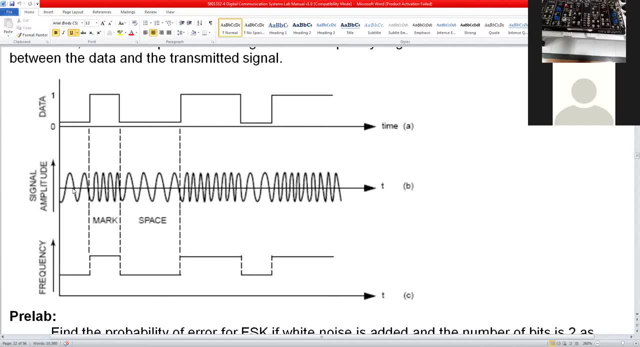 we have seen that frequency can be modulated. frequency can be changed. as you can see, a zero is modulated by the low frequency and the binary one is modeled by the high-frequency. the high frequency, where the binary one is modeled, is called mark frequency and the zero of that particular data pulse where the zero is being modeled. 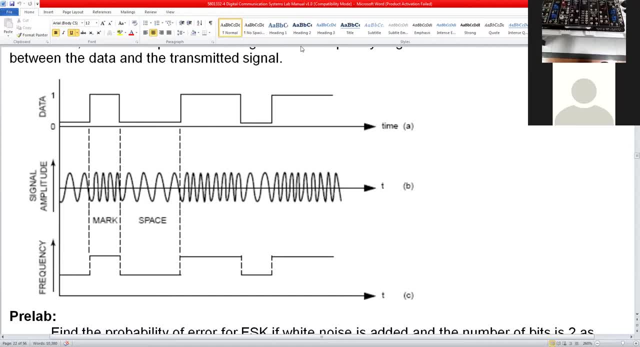 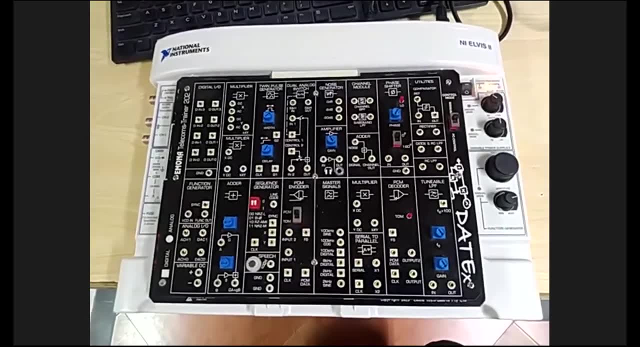 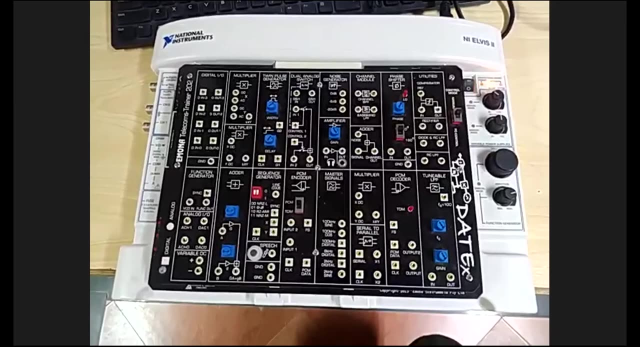 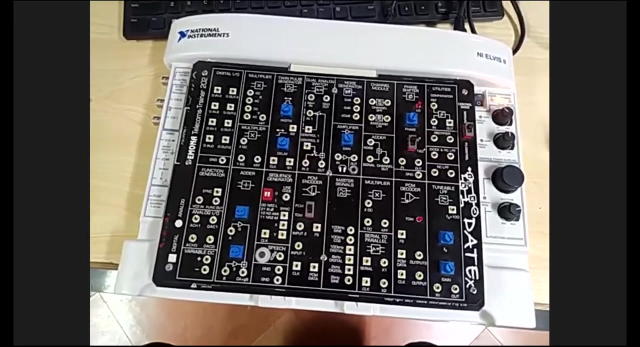 that is being termed as the space frequency. these are the two terms, these are the two things which make fsk so which which is basically a modulation scheme which is used to send digital information between digital equipment such as computers, teleprinters or some other computing equipments, so the data is basically being transmitted by a 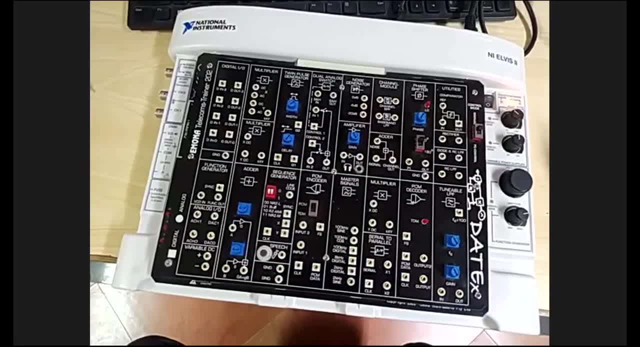 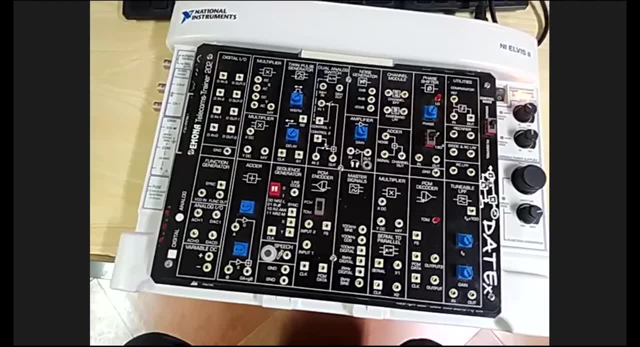 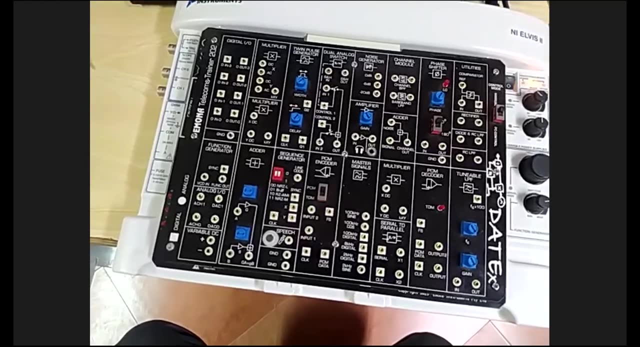 shifting of the frequency of a continuous carrier which i was talking. the carrier is continuous and that the shifting being taken place in the frequency domain of the frequency is being shifted in a constant manner either. for representing zero, we have got a. we have got a definite low frequency. 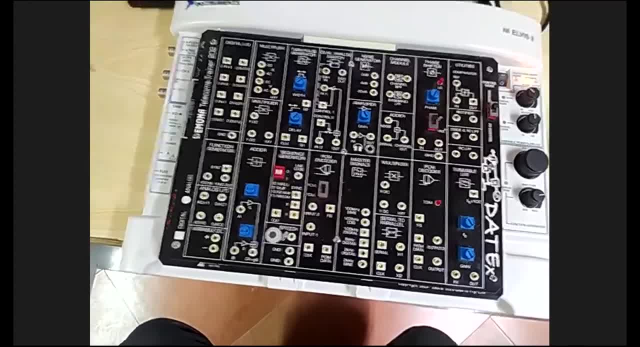 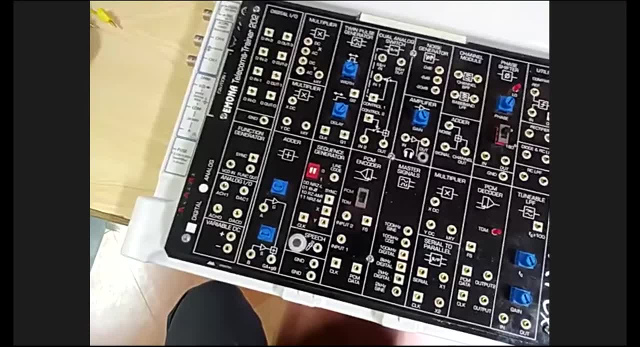 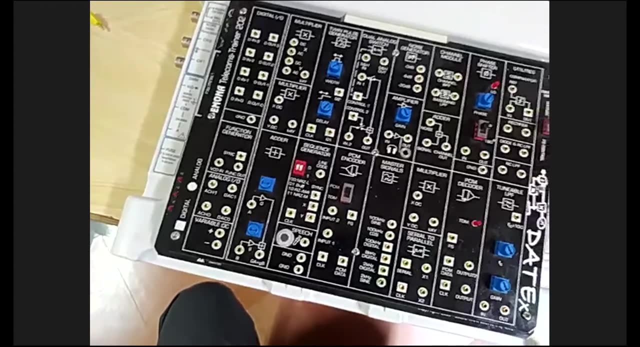 and for representing the binary one, we have got definite high frequency, which is can be marked as a mark frequency, and the space frequency by convention mark corresponds to the higher body frequency and the vice versa. so what we will do, we will use this ni ls2 powers board for the fsk modulation. 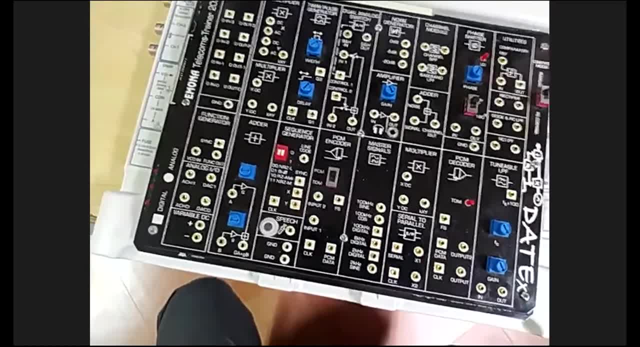 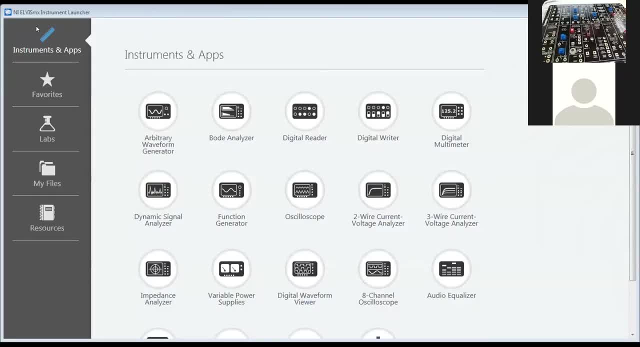 now we will start the ni ls board, the lab of this, and on this ni ls board. so basically this ni ls soft panel, where we can see different options available, and we can control this ni ls, the hardboard, the hardware, with this soft panel. so we'll be using a 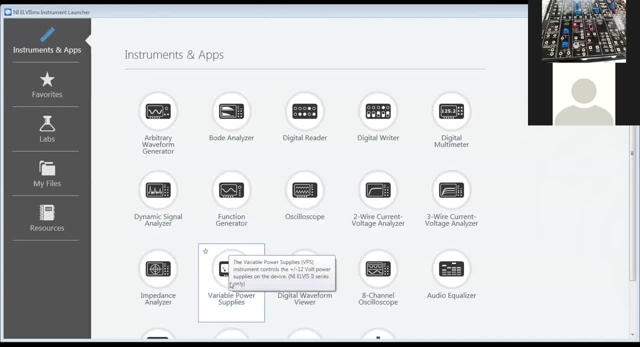 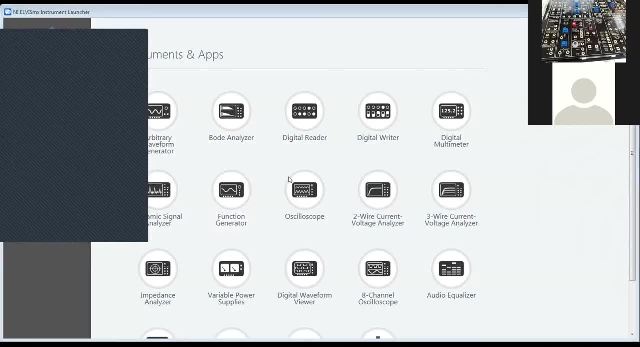 function generator, oscilloscope and the variable power supply. i will double click. the function generator will open. this is how the function generators- function generator or slow scope. i'll share the complete score so as the model when we map the variable operating himself, and i can also. 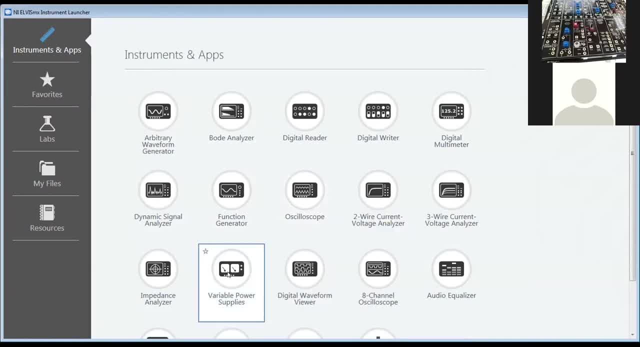 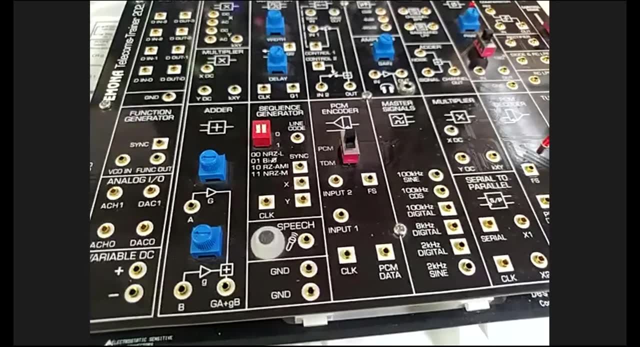 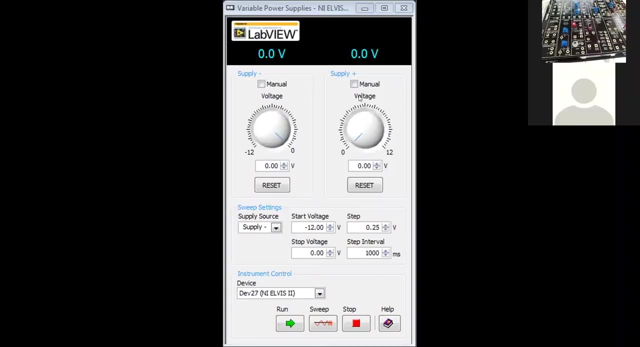 screen so that you can also look these different panels. okay, so let me share the screen as well. let me share the screen as well. this is the variable power supply. this is how the variable power supply looks like. we have got positives, positive- sorry, positive- and negative, and we will we, if we want to change. 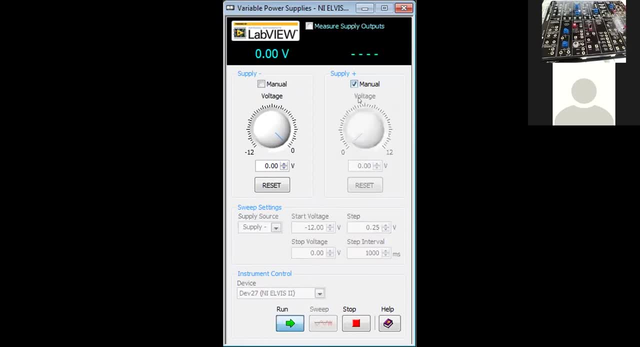 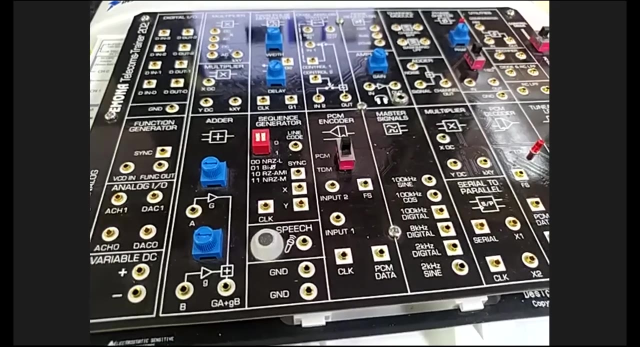 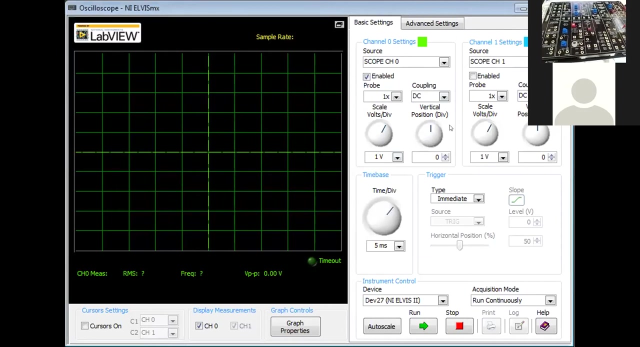 first press the run button and you can see when i change the value of the positive voltages changes. second, we have got sorry. secondly, we have got the oscilloscope. this is the oscilloscope which is being presented over here. we have got very same knobs and controls as we have got in the hardware section. so now, 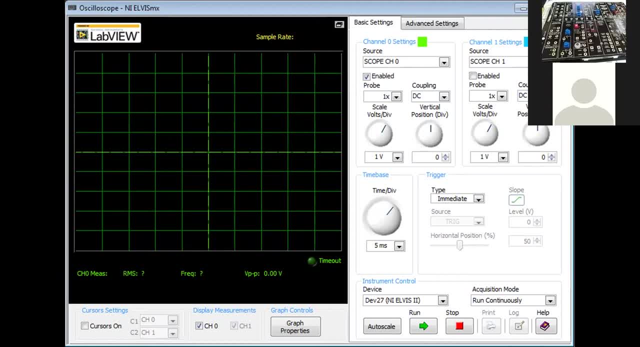 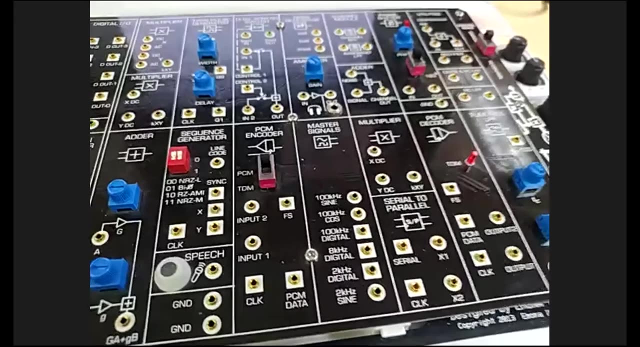 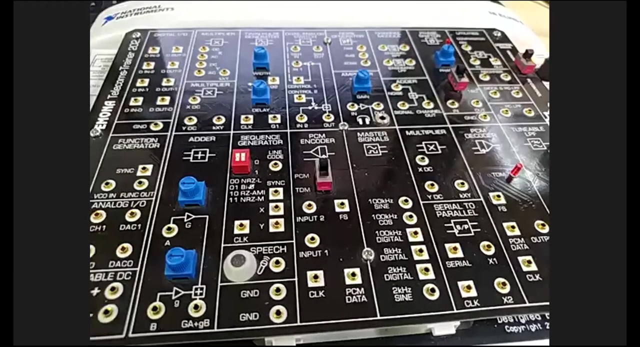 we'll, we'll, we'll, we'll- going back to the topic again and see how we can learn and how we can see different aspect of this: frequency phase shift. frequency shift: okay now. okay now. first of all, we need to adjust the function generator: use specification and when. where i can find the function generator, let me share the screen of the. 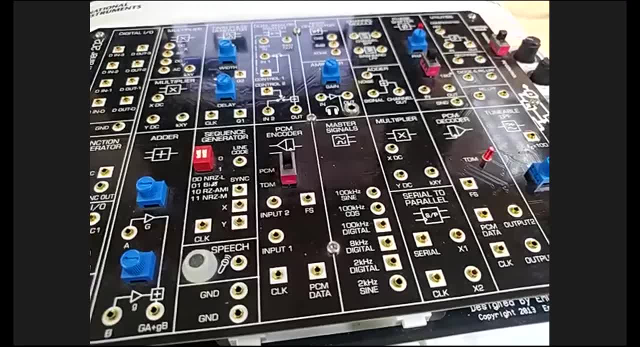 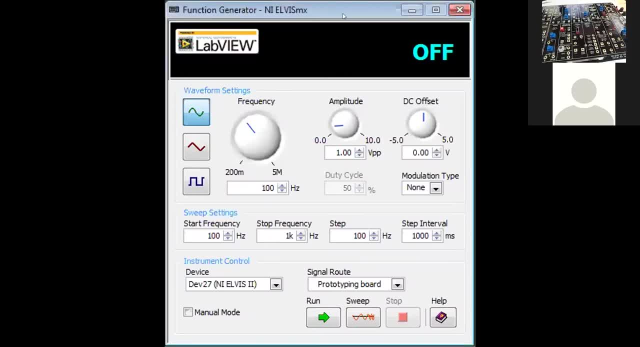 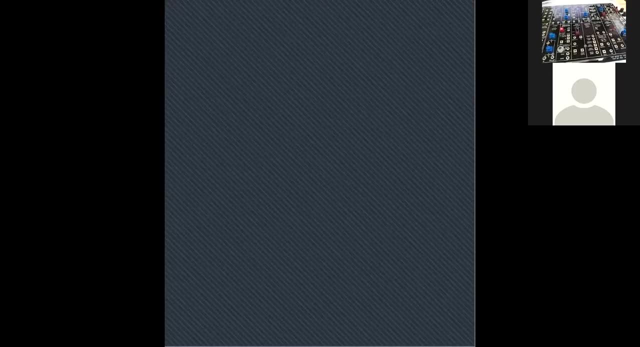 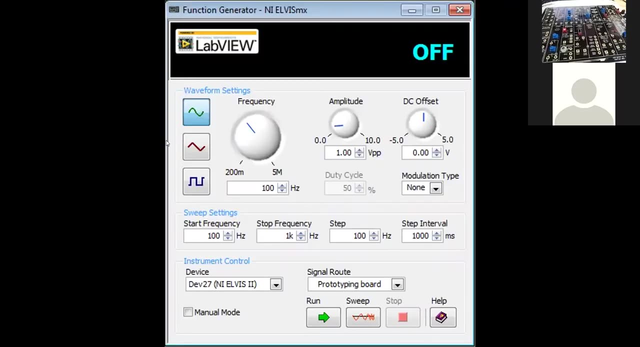 function generator for you, for you, human launcher function and in this function generator- okay, there is the function generator. you can see the function generated. the function generator must be modeled, which have, which should have, wave as a sine wave, sine wave. yes, we have got two waves: one is sine, the other is triangle, the third one is square. 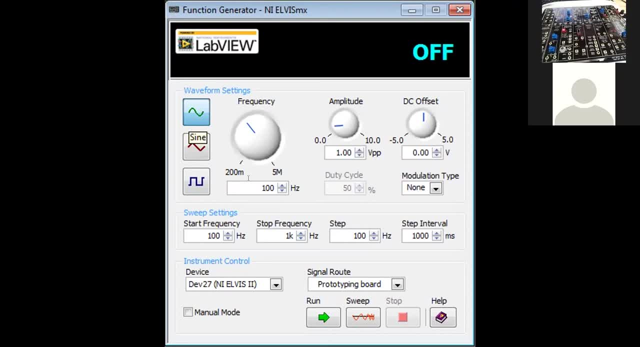 so we should select the sine wave. first the frequency must be 10 kilohertz. so 10 kilohertz means we should have got 1000 and then 10 000. this is 10 kilohertz. amplitude is 4 volt. this is 1 volt. 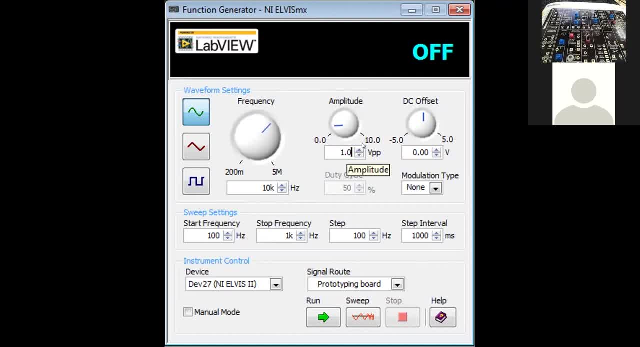 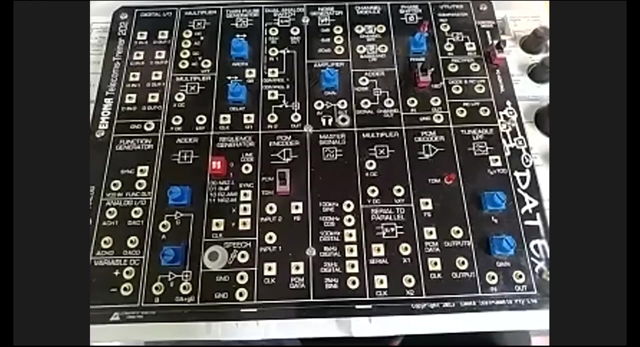 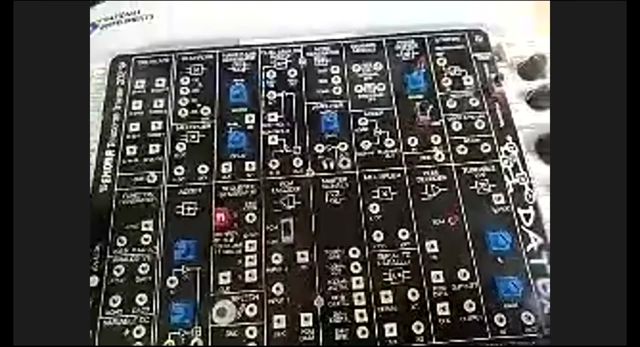 sorry mistake, should. this modulation type must be fm. the modulation type is fm and this is how we can connect the which. this is how we can set up the function generator. okay, okay, okay, okay, okay. now we will connect the diagram as per the diagram, the master signal. we have got the master signal. 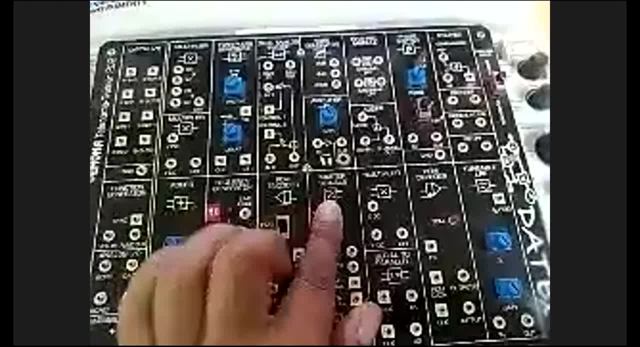 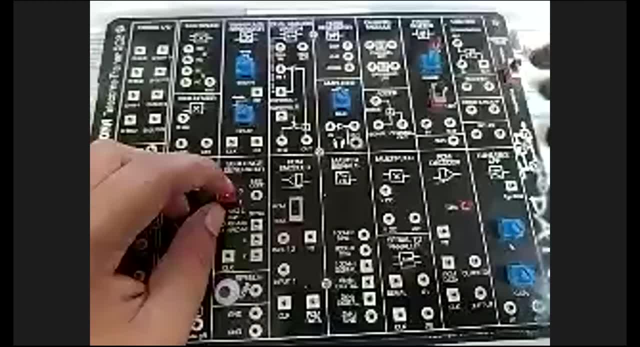 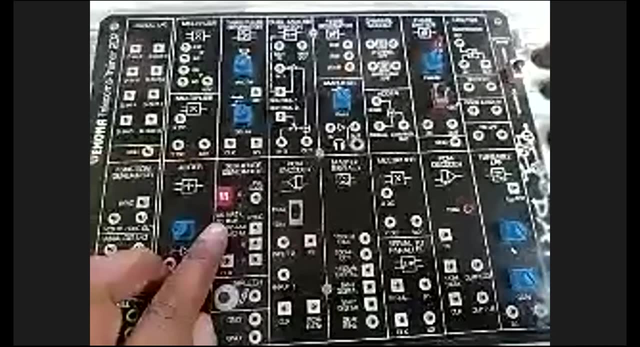 over here. this is the master signal. the other one we will be using is a sequence generator which is over here. the sequence generator- sequence generator has got two soft dip switches. if you've got, you can see over here. double zero represents non-return, non-return to zero. the 0, 1, 1, 0 and 1: 1 are the. 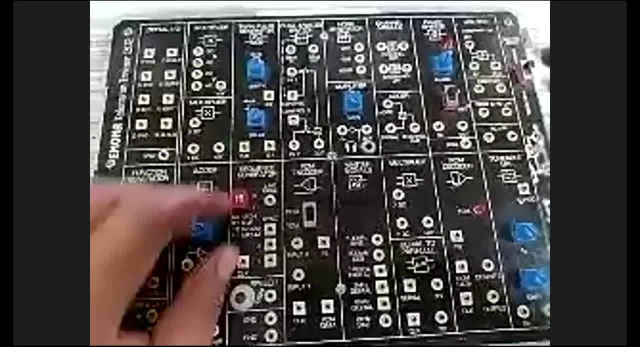 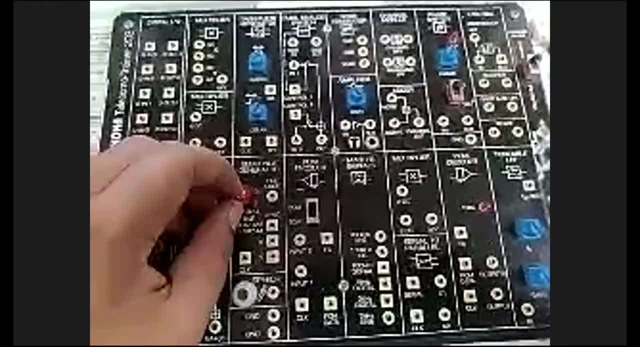 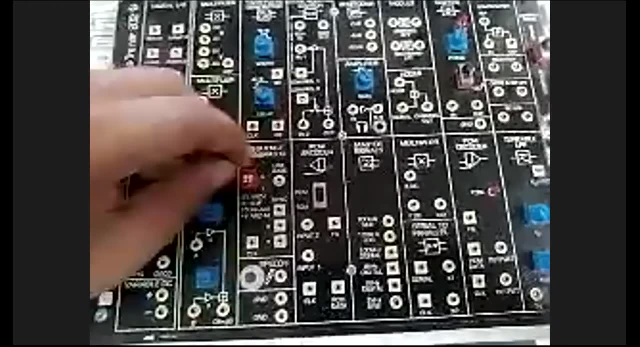 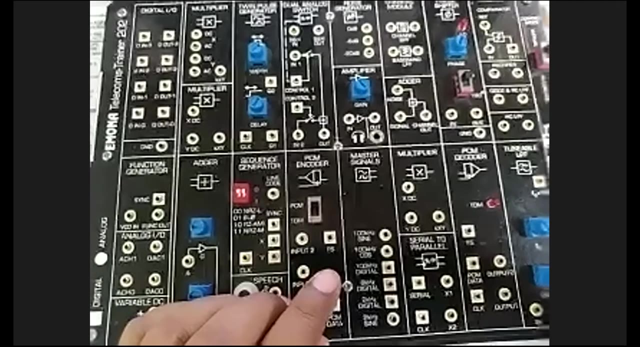 different line coding, line coding schemes that we can utilize. so, for instance, this is zero, sorry, this is 0, 0. and then if you select the dip switch or the slider, this dip switch, on the downward side you can say: it's 1, 1 now, so dip. 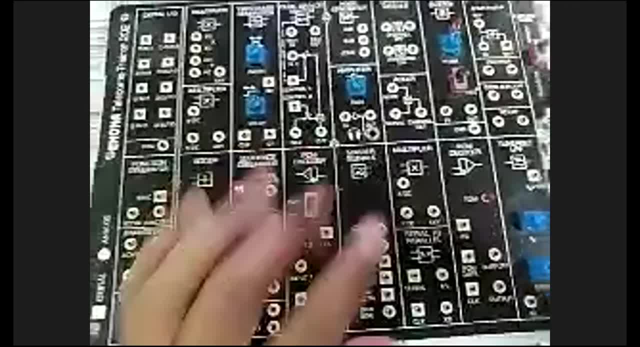 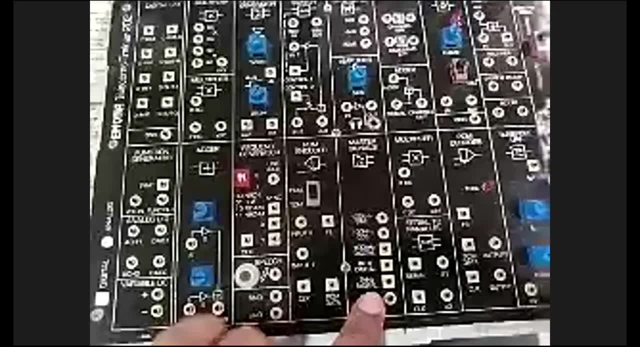 switches can select different line coding schemes. so basically, to set up digital sine wave, two kilohertz- sorry, two kilohertz- a digital wave, and we will use this two kilohertz little wave to clock the sequence and this the line code and the sync pulse. 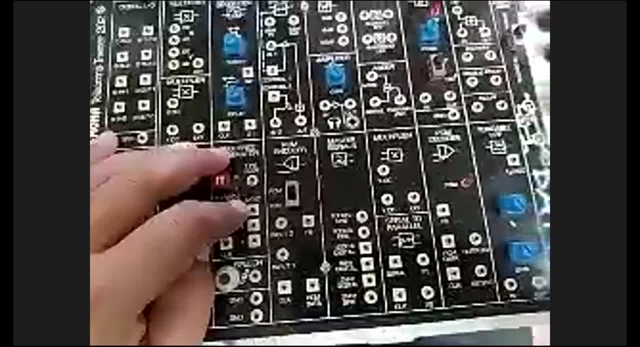 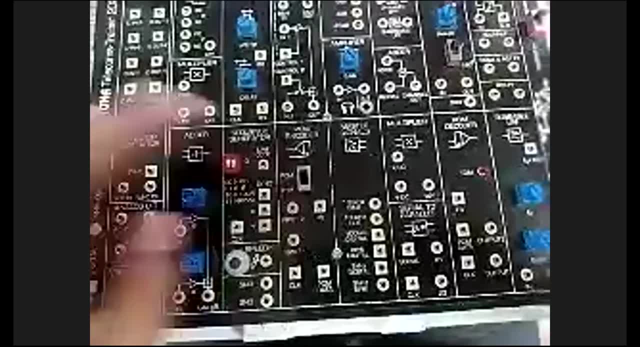 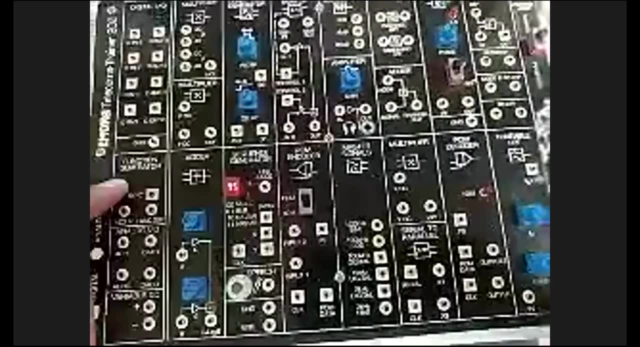 will be used and then this sync pulse will be observed at channel zero and the line code output will be utilized as the function generators inputs. okay, this is the function generator over here, the function generators inputs to the voltage control oscillators input. so we will be giving, we will be giving line codes input to the vcu in so that the vcu can oscillate. 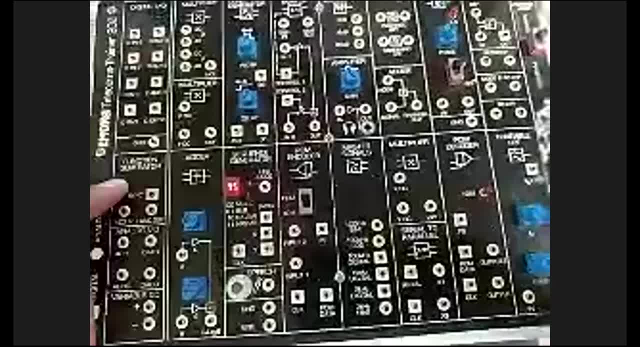 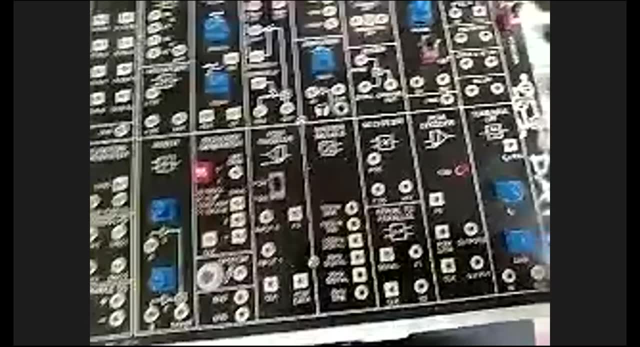 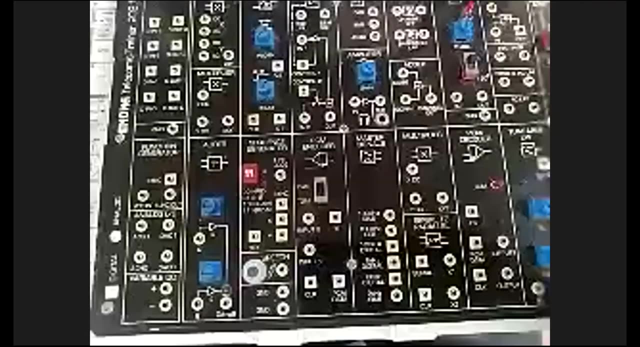 at the frequency being generated or the voltage levels, not particularly the frequency, but the voltage level- from this line for the vcu, and then this function out will be observed at channel one. okay, now hard wiring the lab. first of all, as per our discussion, we will be using the master signal of two kilohertz digital wave, okay, and this master will be 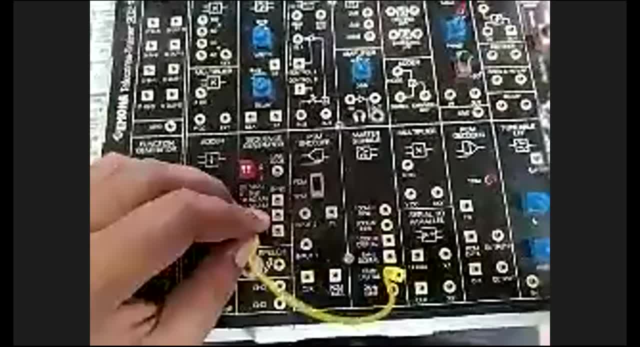 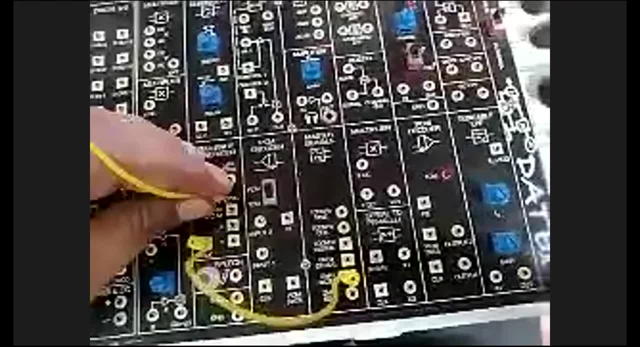 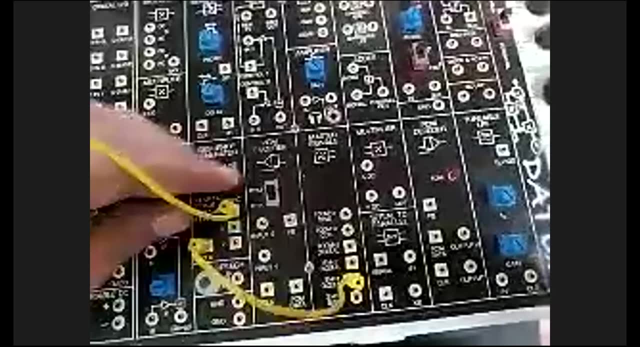 used as the clock frequency, and then we will be using the sink pulse from this sequence generator- see the sink pulse. the output of this sink will be used to the frequency generator. so then, Does This how we plugged in? we have got three leads over here. 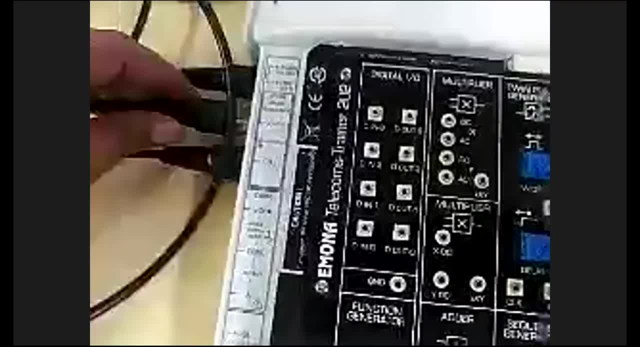 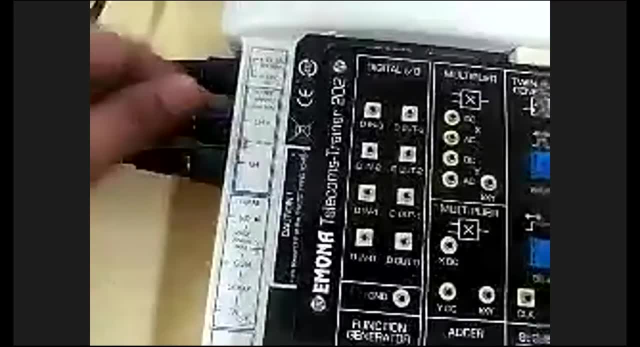 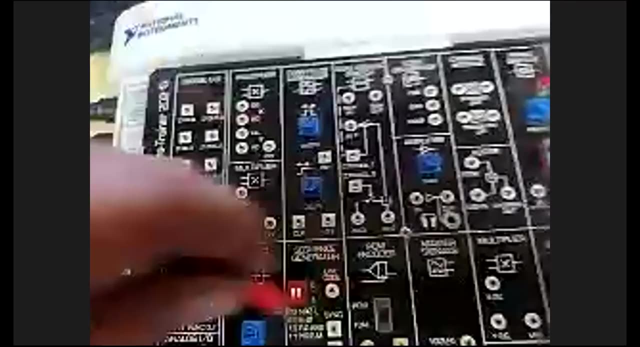 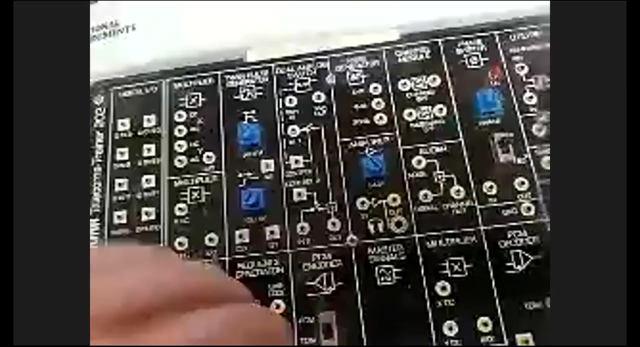 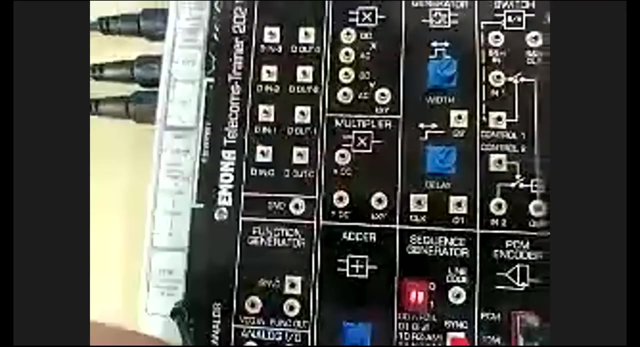 the lead is over here. this is how we plugged in. this is the channel zero. okay, now these are the clips and then this will be going into the function generator sync and then the ground over here. okay, see, i've connected. okay, one thing that i've been taking. 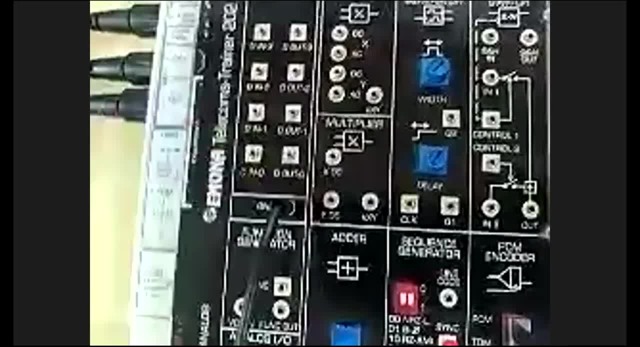 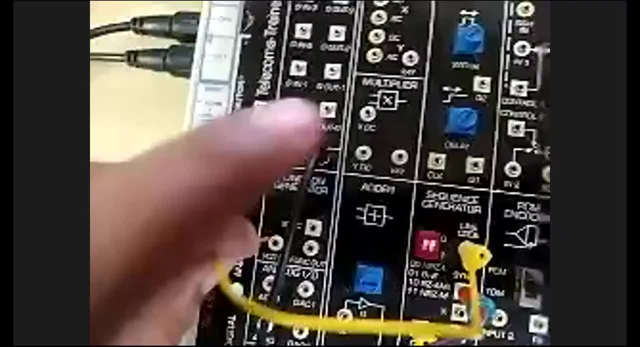 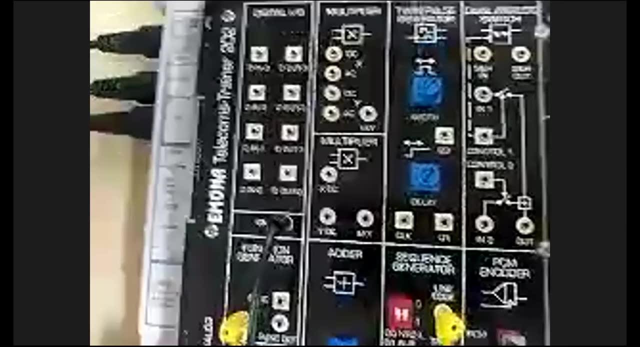 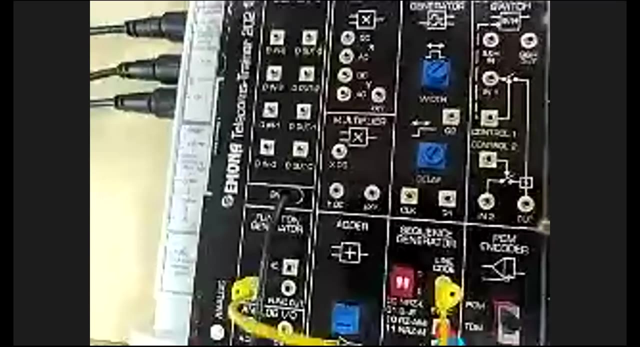 not properly been done. okay, now insert it properly. line code will be taken as the voltage control oscillators input and then it is then dusted, the line line code. the output of the line code will also be observed at channel zero. the channel zero is here: channel zero. sorry for the shaky video, because i'm handling the 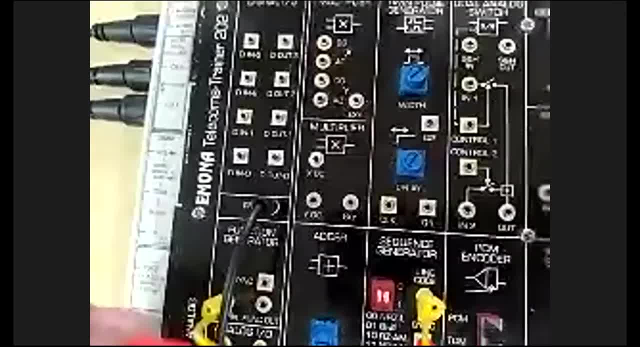 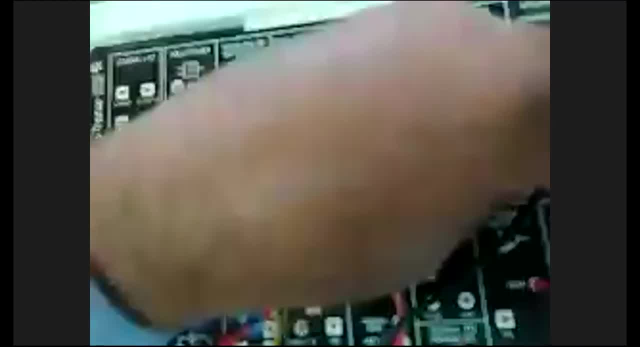 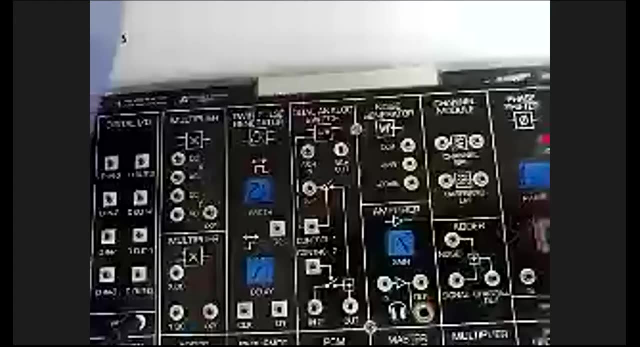 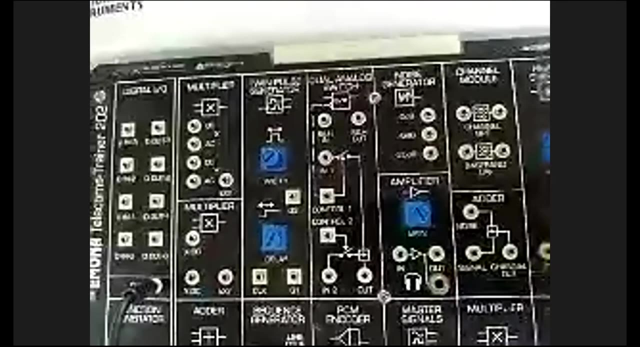 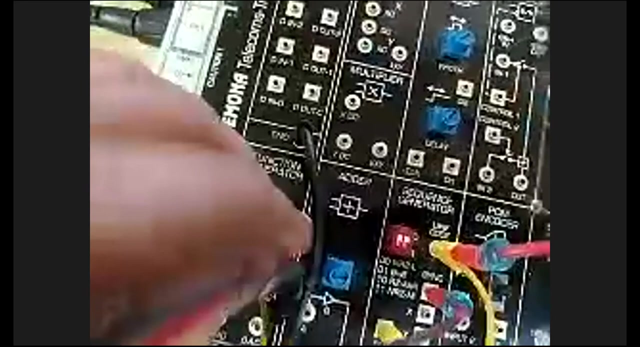 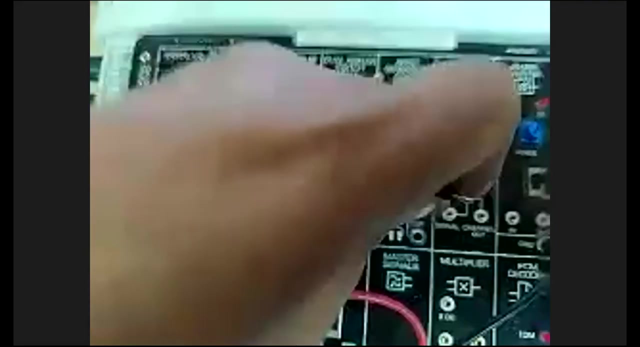 camera by myself. okay, line code and then the ground. there are multiple grounds available. get around over here: the line code being observed at channel zero and at channel one. we will be observing the function out. this is the channel one function out. the trickiest part is just to find the ground. 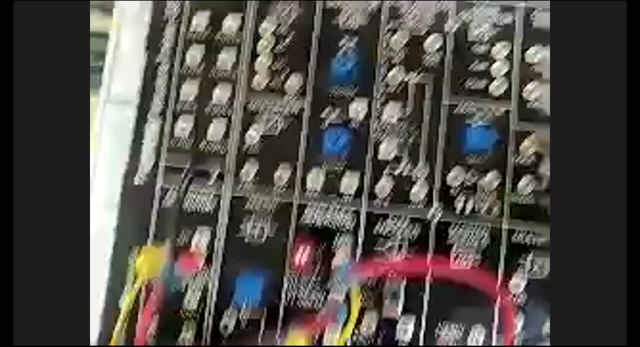 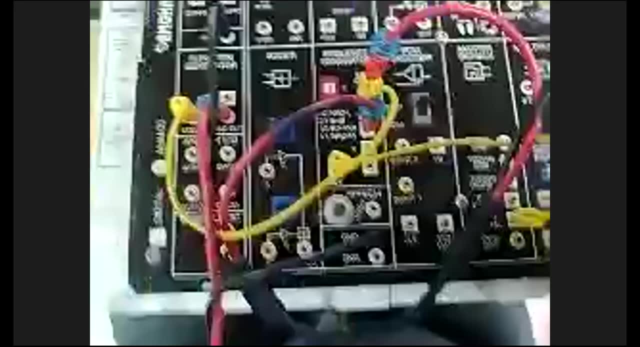 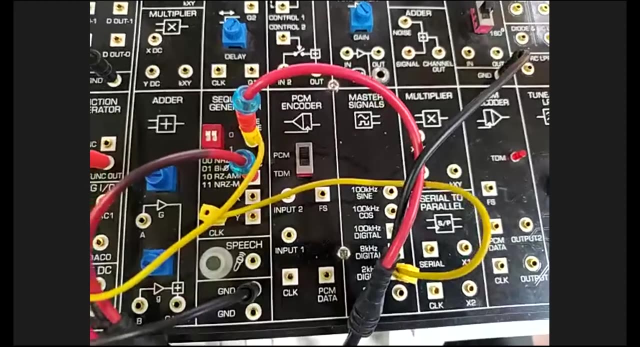 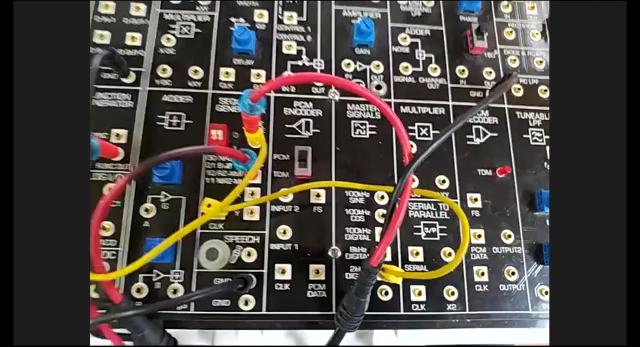 i'm something, okay. okay, see, now the wired has been, i've been plugged, okay. first we will launch the detect soft front panel, sfp, sfp, and check that you have soft control over theono data experiments so you can easily locate some soft buttons on the. 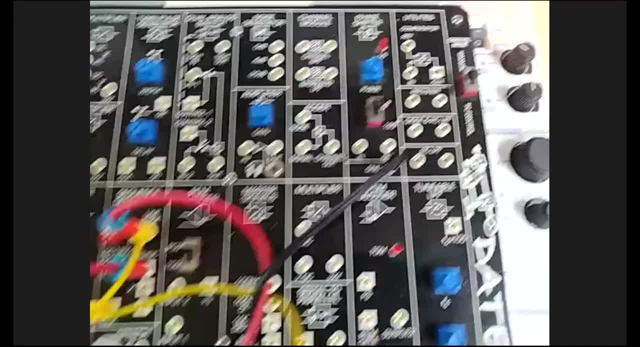 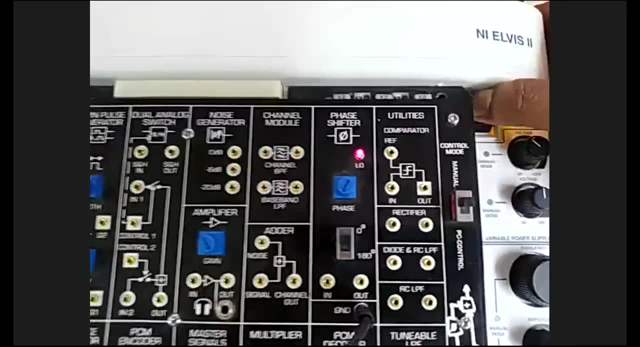 emono data export over here. we have moment DJI x Waterboxx- Dć Ск má bứá, something here. we have got power button. if you turn on, the green led will turn on and then another main power switchboard is over here. this is the main power switchboard. you can easily see this. this is the 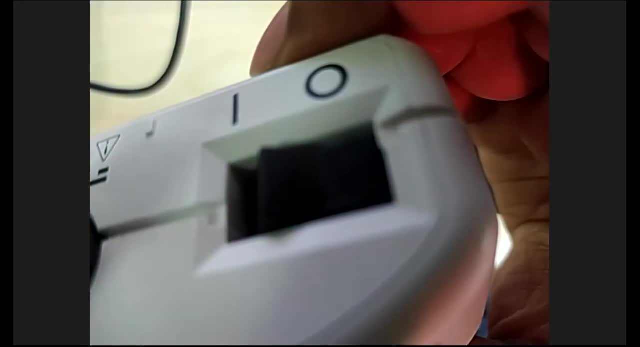 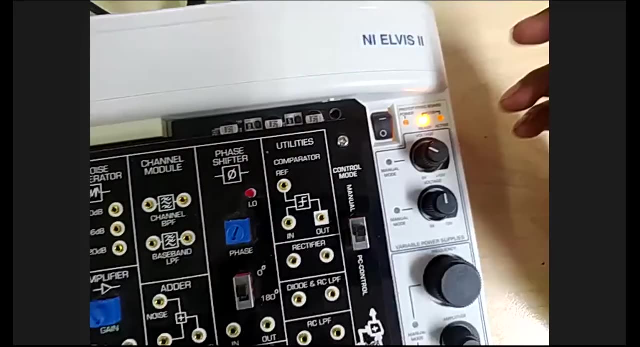 main power switchboard. this will turn off the monodetex board and this will turn on the immuno detector. so this is the main power board and this is the soft control board. okay, these are the two switches and if, when we turn on the power of programming mode, this will turn on the leds. 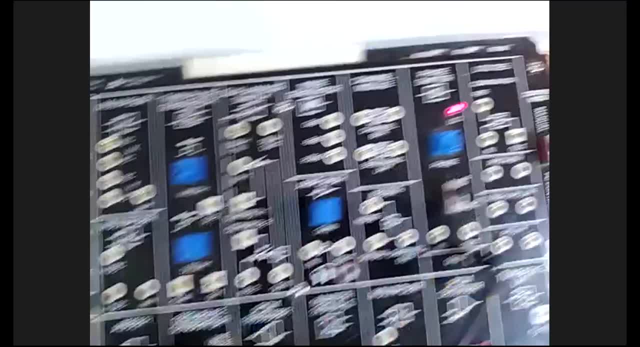 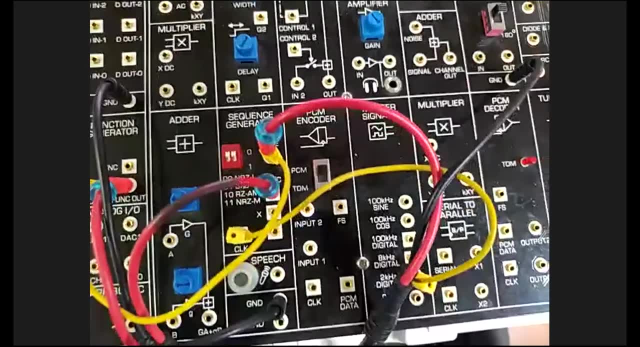 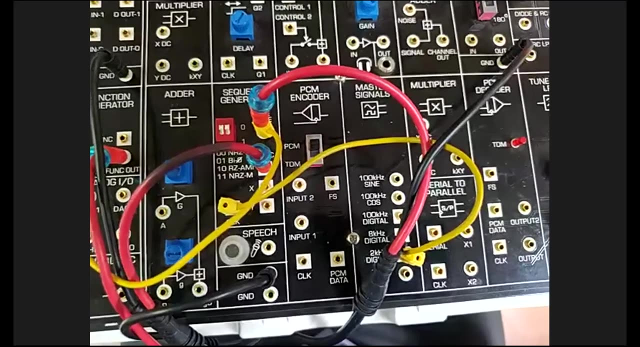 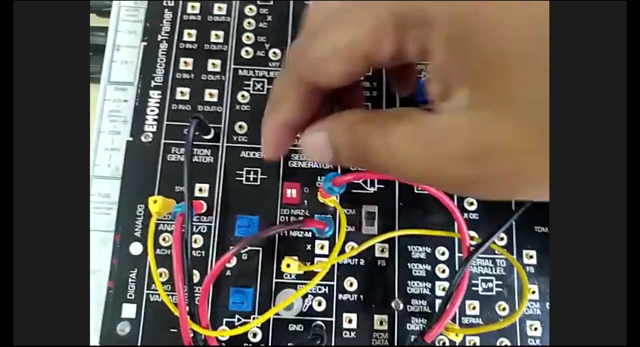 and these three LEDs over here. okay, now since we have got the soft control over the immuno detect export, we will launch and the soft panels sequence generator module and set the soft switch or the two dip switches to the zero zero position. this is as previously i have said. 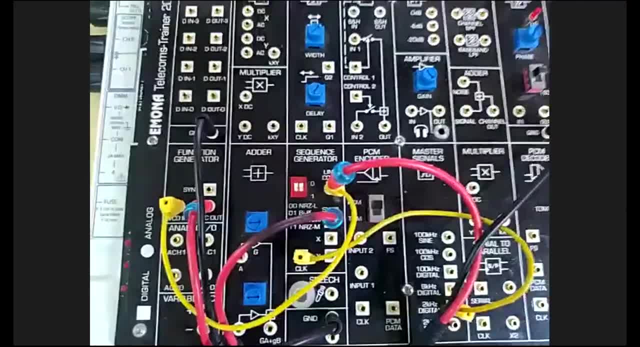 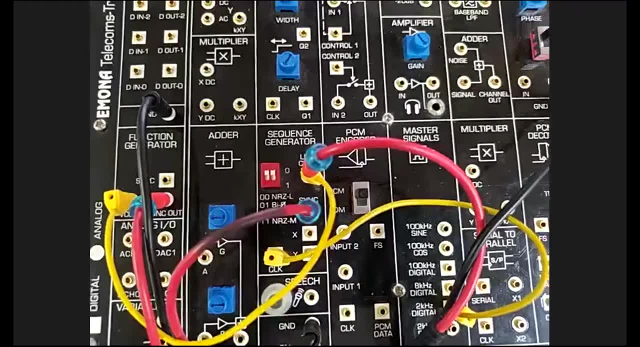 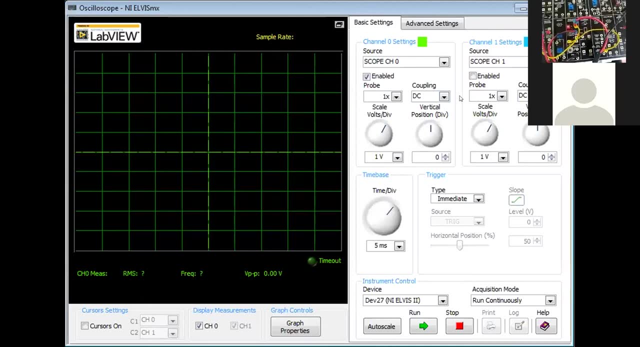 this is one one and this is zero, zero. i've turned the soft dip switches to zero, zero and then i have to run the ni elvis scope board or the score oscilloscope. activate. activate the scopes channel one. now the channel one is activated by clicking this enable. 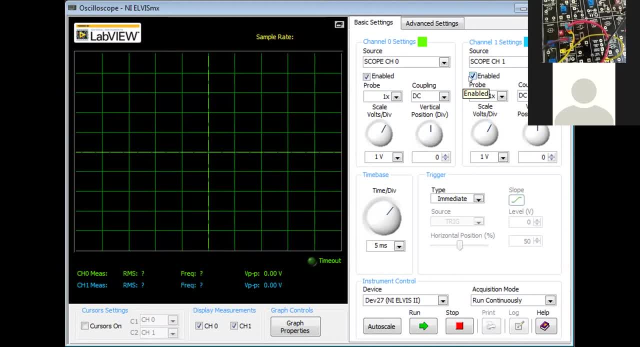 button you can enable or disable the given channel or the or the stated channel. activate scopes: input to observe sequence generator, modules output and the fsk signal out of the vco, since we are not getting any output because we haven't connected the board yet. so first the board has to 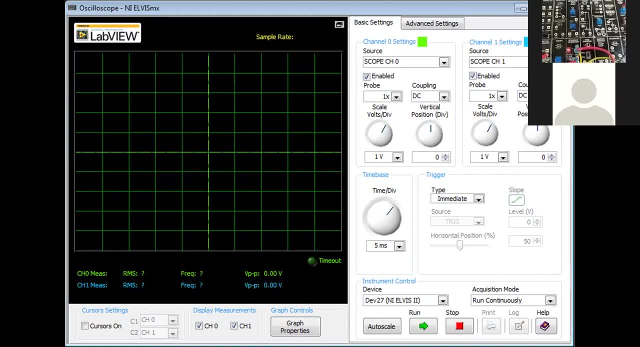 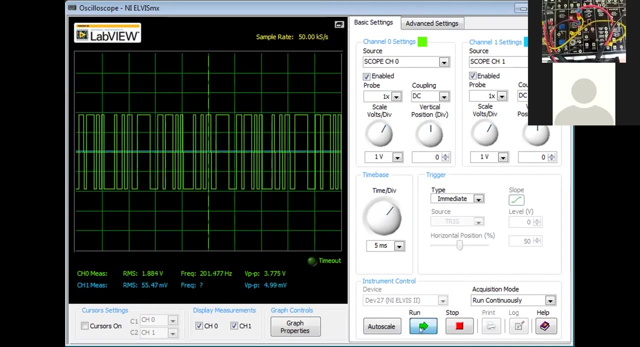 be connected and then, sorry, the board. the signal has to be as the given as the input. so when we turn on this switch, the board is now activated. okay, so we have got. we have to run. now you can see. so you have to press the run button over here as well, so you can see the output of the sequence. 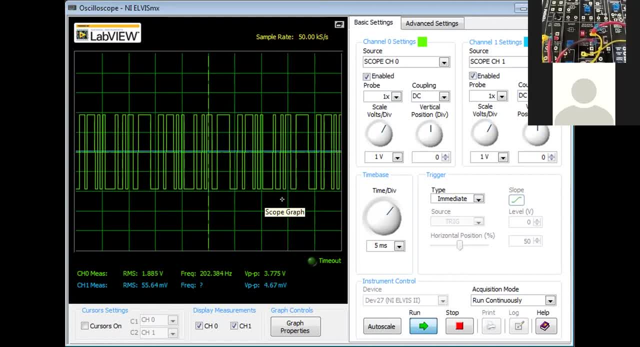 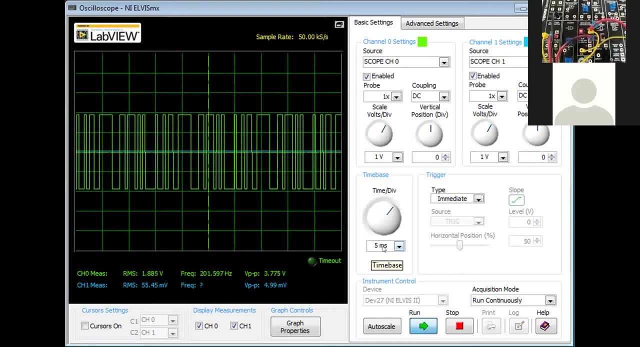 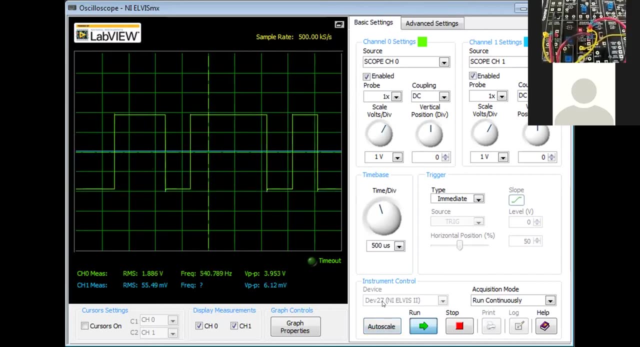 generator module, the fsk signal out of the vco, so ensure that the scope's time base is at 500 microseconds per division. this is the scope's time per division: 500 microseconds per division position. okay, this is the part one of the lab that we have performed. now moving to the part 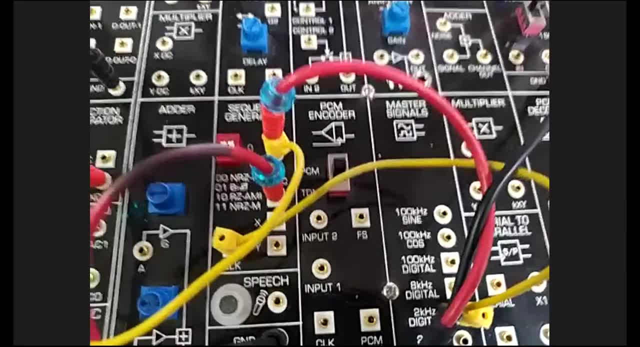 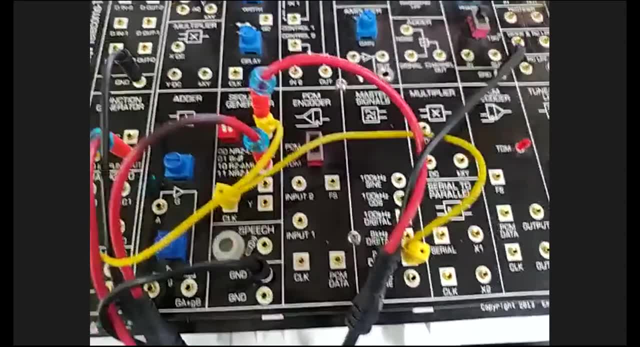 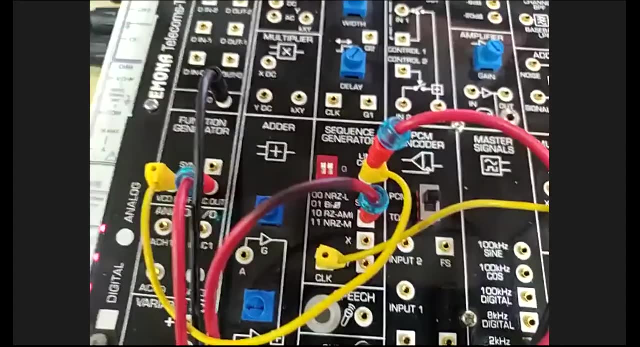 two. part two or the part b is the demodulating, or how to demodulate an fsk signal using filtering and an envelope detector. as fsk is really just a frequency modulated with a digital message instead of speech or music, it can be recovered using any of the fmd modulation schemes. however, the fsk 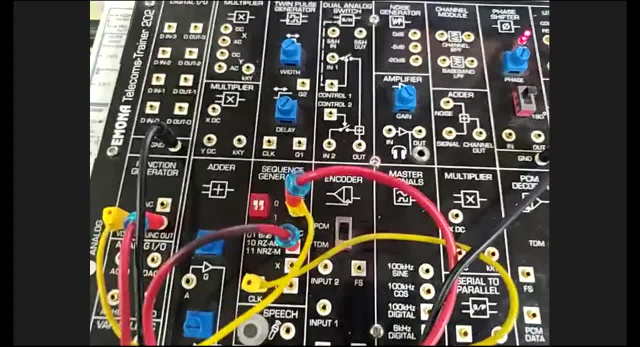 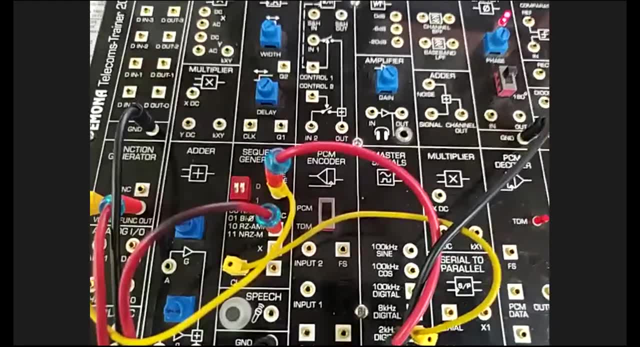 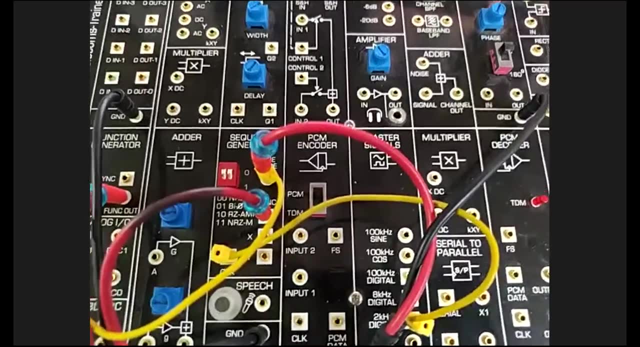 signal switches back and forth between just two frequencies, we can use a method of demodulating it that cannot be used to demodulate speech input fm signals. so the next part of the experiment is to demodulate an fsk signal and then we will hardware the spider, as per the experimentation. 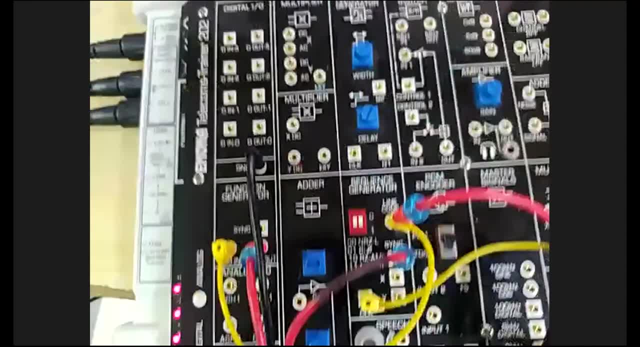 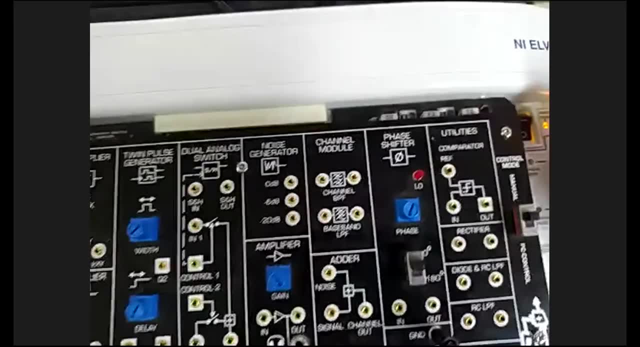 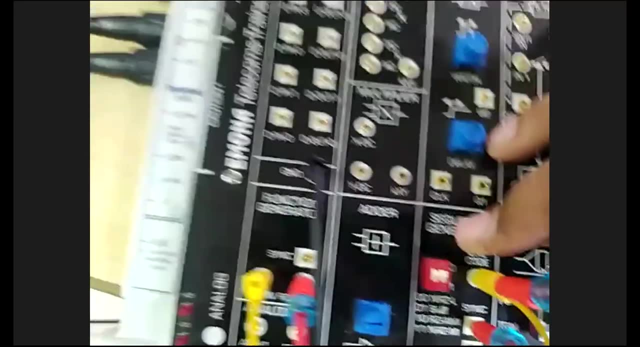 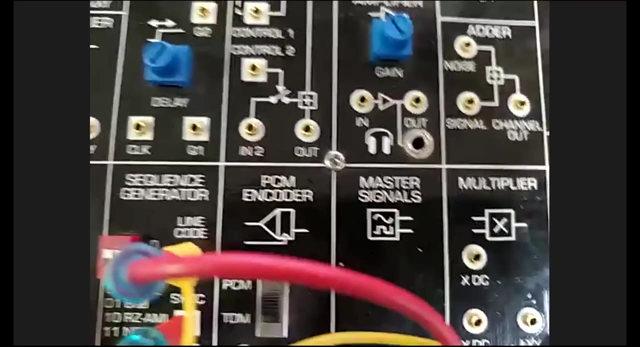 okay, for this we have previously utilized the master signal sequence generator. okay, first turn off the switch so you turn off the board over here you can see the board is being turned off. so we have utilized master signal sequence generator and the function generator. now for the demodulation, we'll be using team tunable lpf low pass filter and the in utility section. 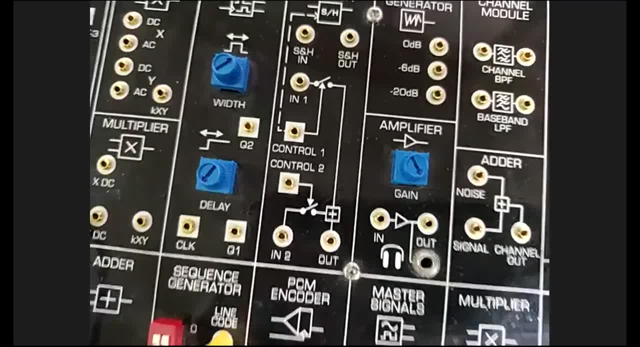 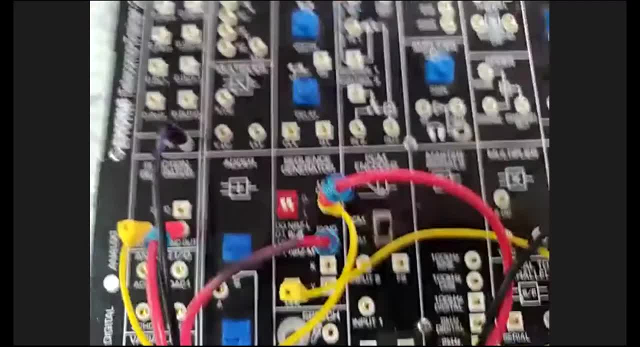 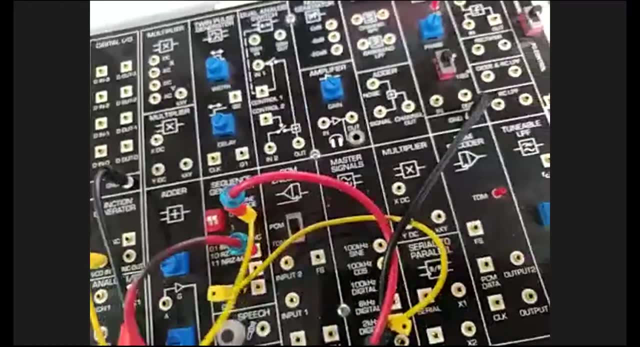 we'll be using diode part or diodes part and we'll be observing it at channel number one. so okay, now hard wiring it. first of all using the function out, first of all using the function out over here plugged in, plugging in function out to the tunable. 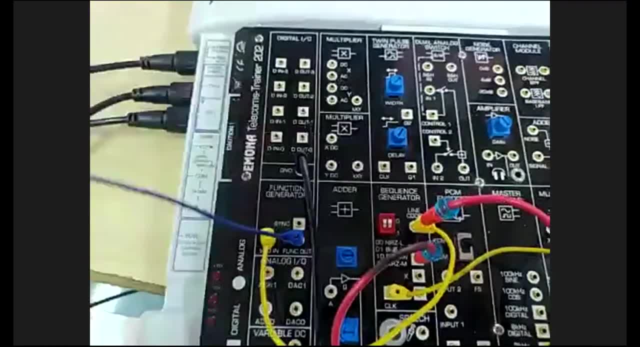 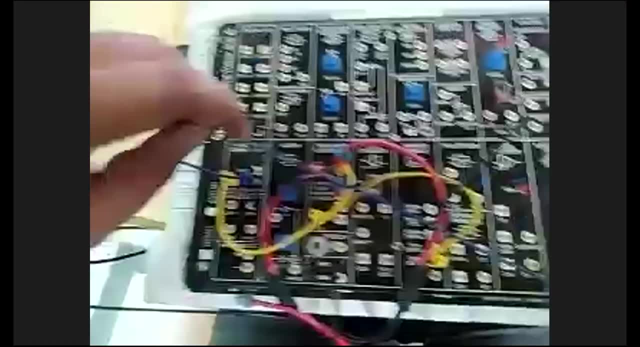 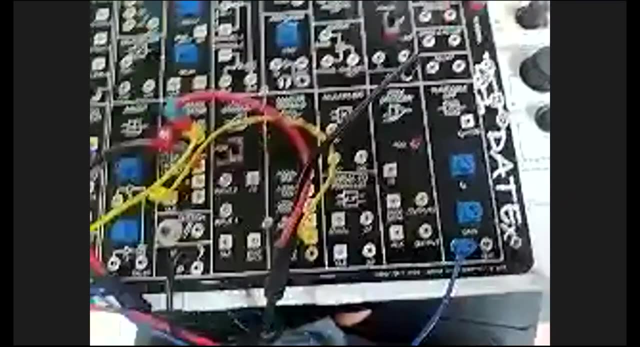 lpf. okay, see function out to the tunable lpf and then from tunable lpf we have got another port of output. from this output we have to connect channel number one. this is our channel number one. so we are going to connect channel number one to our channel number one. 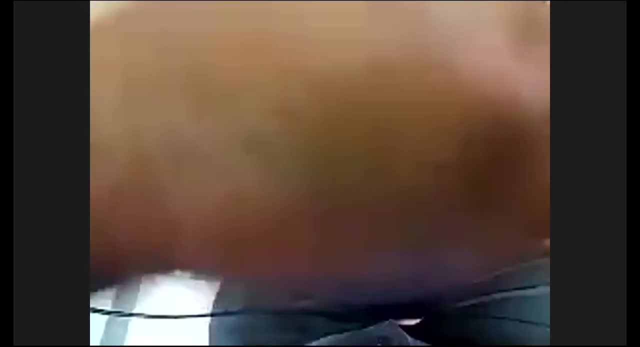 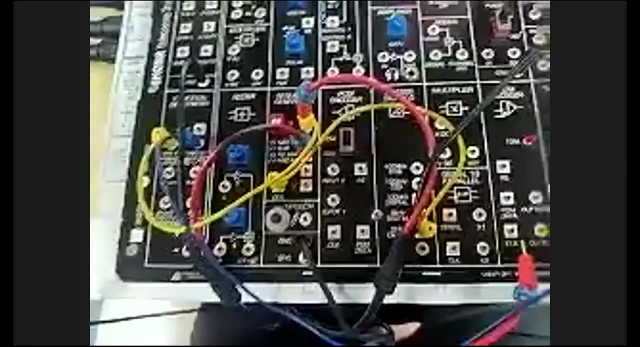 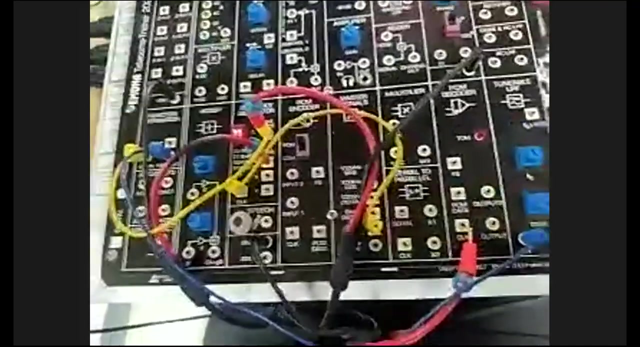 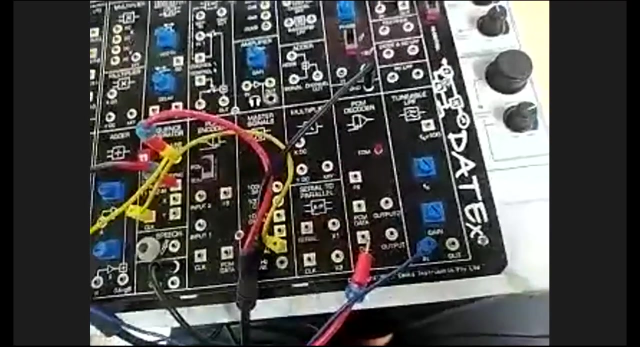 the channel number one. okay, here we go, the channel number. when we connect it, the function out okay. one of one more thing: i have to use the smallest part or the smallest wire. i'm just get it okay. now i've got the smallest one. okay, from the function out connect. 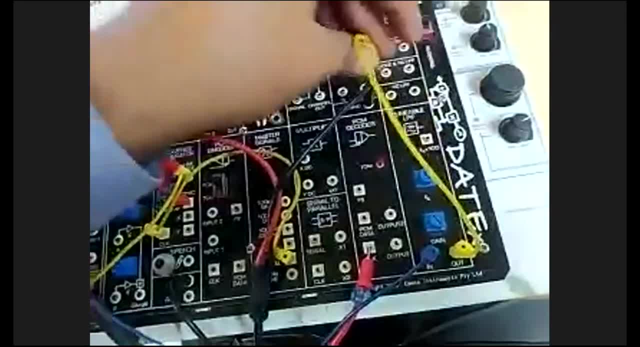 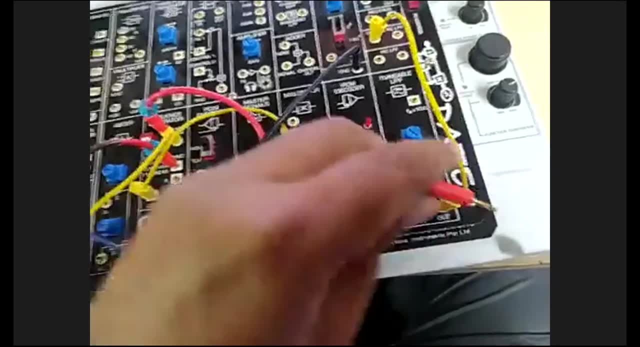 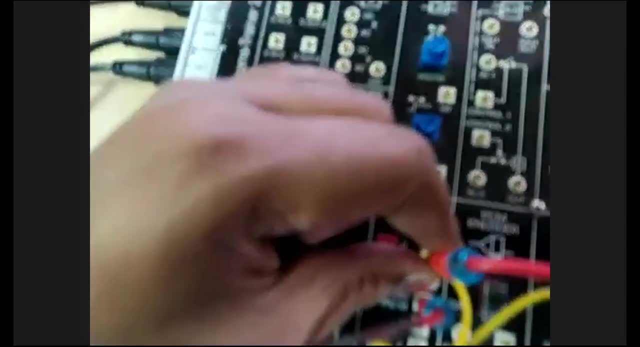 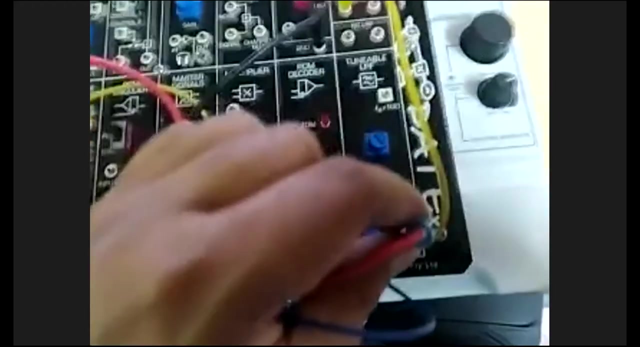 on the function out connect is diode filter, okay, and then you see this function out over here. so again, at channel zero will be. we are observing the line code at channel zero, at channel one will be a channel one- sorry, a channel one- will be observing the output of the data export. 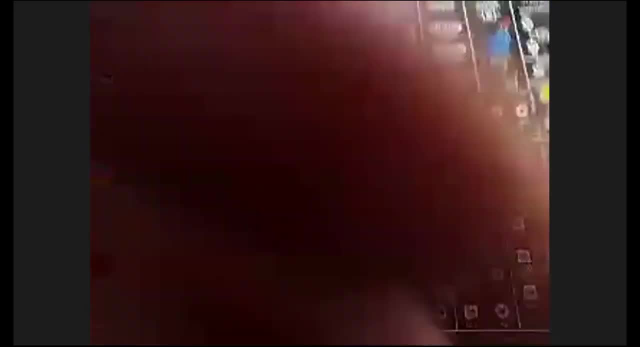 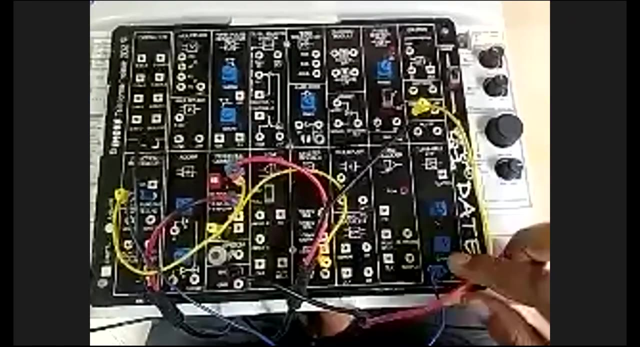 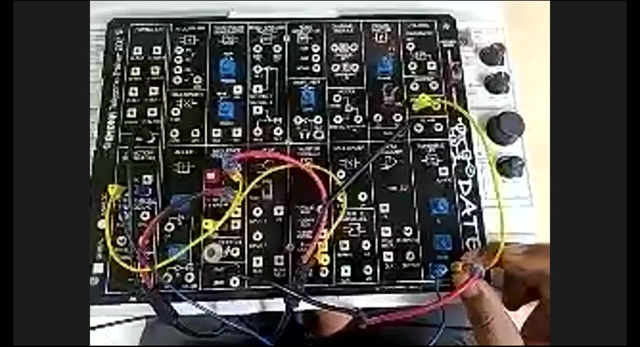 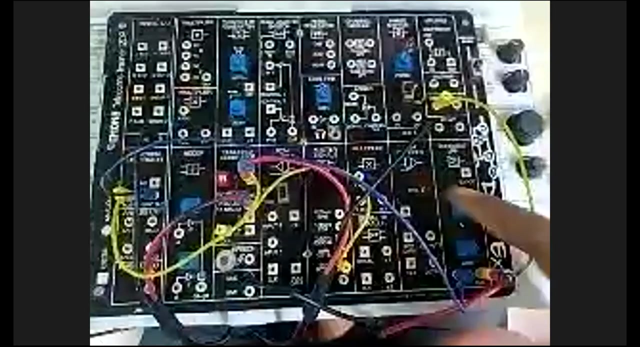 good, good, good, good, good. now again turn. you can easily look the diagrams over here. we have connected this diode to the channel out over here and from in sections. we have connected the function out and then vcu. this is as per the input, this is for the output. we have used the tunable lpf and then tunable lpf. we have got. 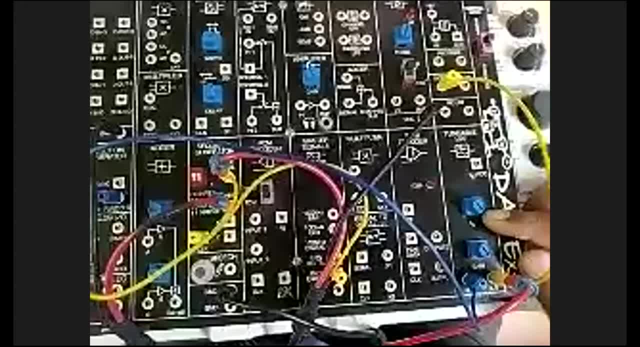 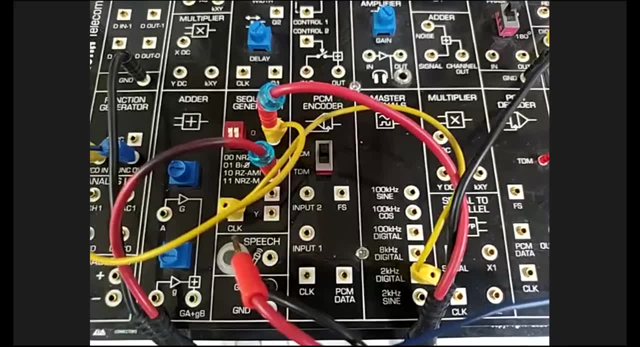 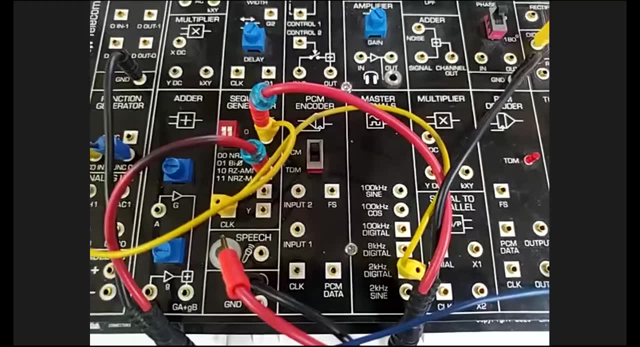 gain and center frequency or the corner frequency. we will adjust this corner frequency and we will look at the results. okay now. okay, now we will back. we will turn on the function generator first. this is the function generator over here. first, we have done all the settings before and then. 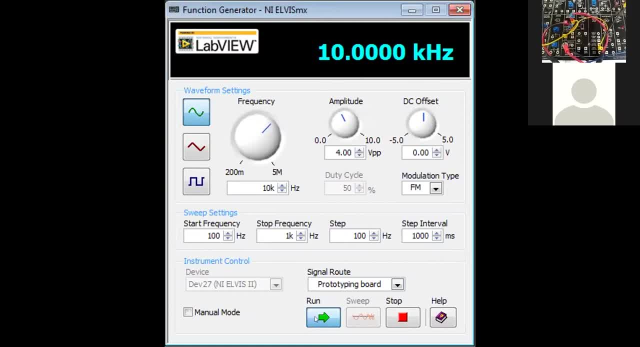 we need to. we need to run the function generator. after clicking the run button you can easily see stop. okay, this is the function generator is on the stop condition after doing 10 kilohertz over here sine wave. 4 volt peak to peak frequency modulation type. 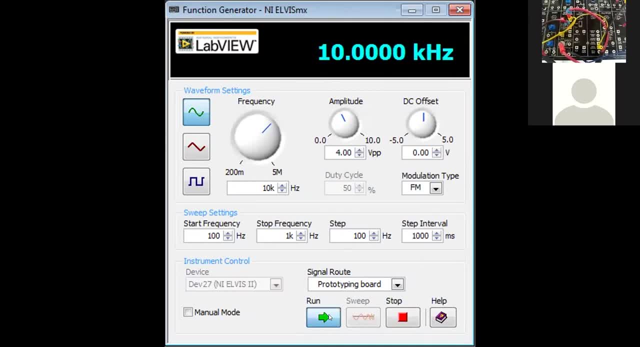 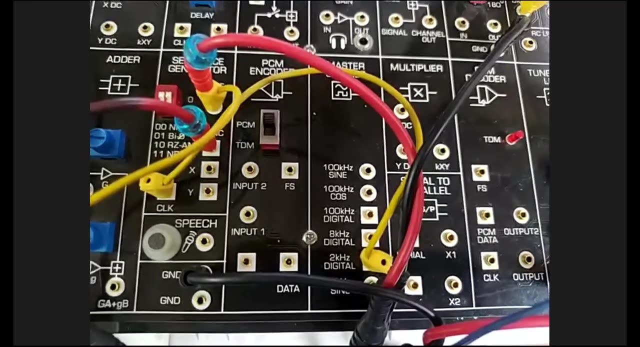 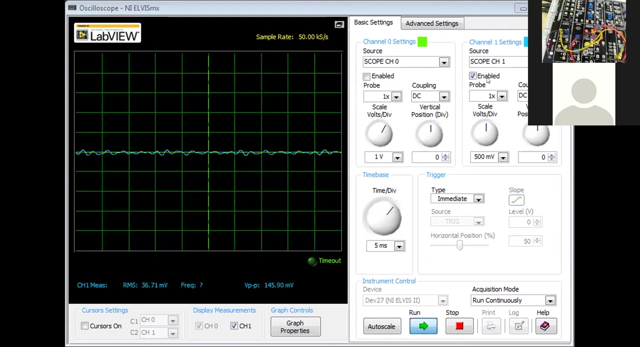 fm or the modulation type fm. click on the run button. when this run button has been clicking, you can easily see. let me share you, let me show you the screen of the oscilloscope. where is the oscilloscope over here? okay, now you can easily see the output and the input, both enabled. 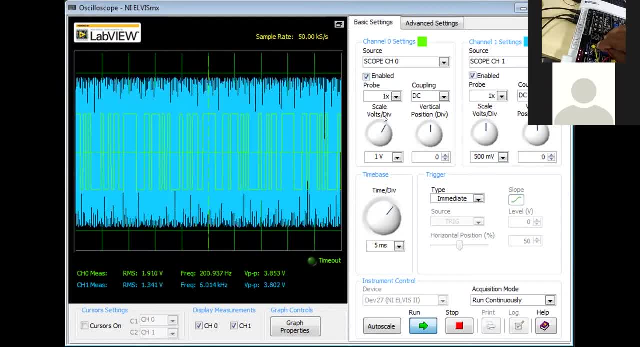 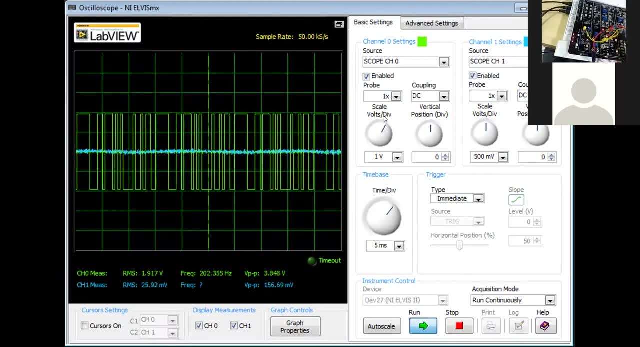 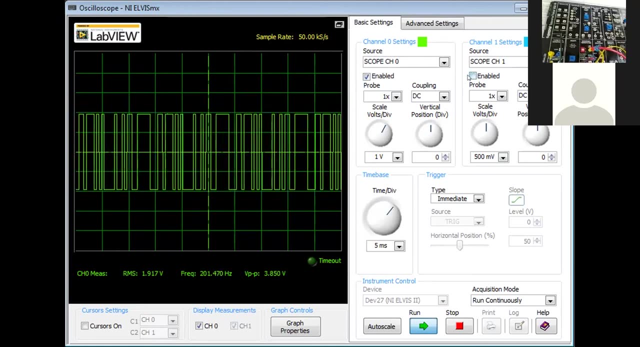 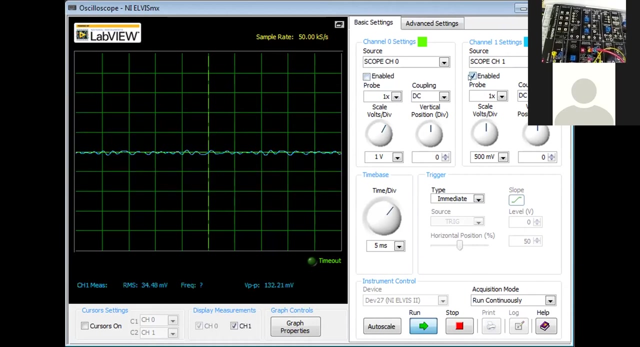 now, this is the input. that's the input and this is the output of the tunable lp. the blue wave, the green one, this green one is the output of the line line code and I will disable this green one. this blue one is the output of the. 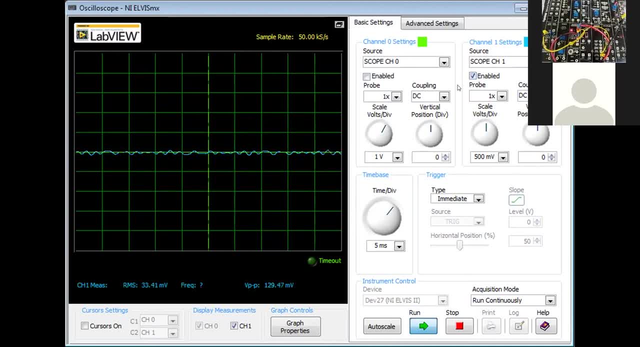 what you can say. the output of the tunable LPF turn, the gain turn, you can easily see on the video I am moving the gain that the one at the LPF LPF over. here I'm on the LP of tunable LPF side. I've got two knobs, the corner frequency. 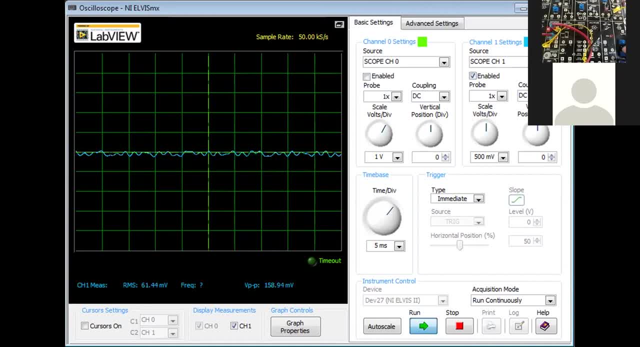 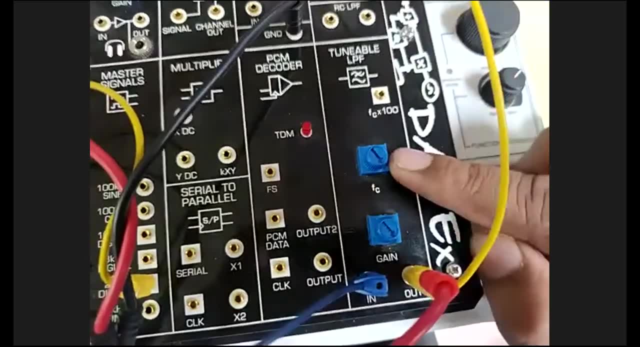 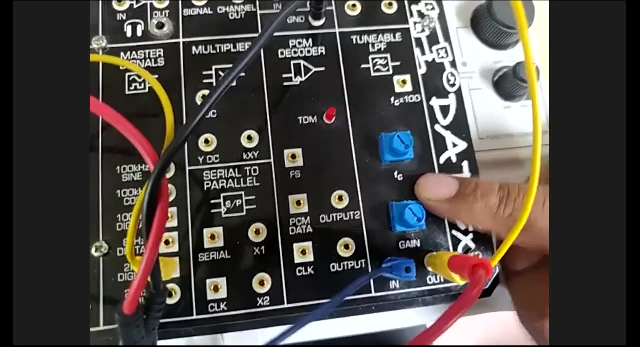 knob and below the corner frequency knob. I've got the gain knob. okay, I will let you know. see, over here we have got two knobs. one is center frequency knob, the other one is the gain knob. sorry, corner frequency knob, corner frequency and the gain knob. turn this gain knob to this position, okay, so that the gain is. 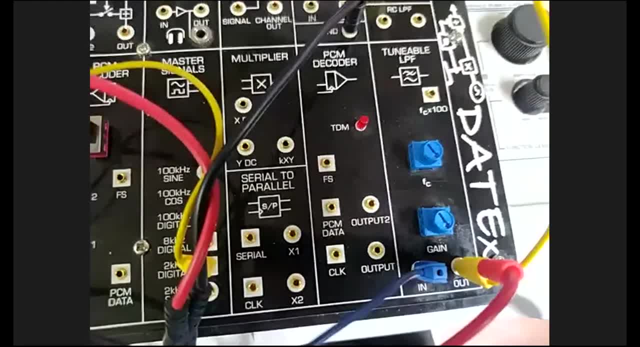 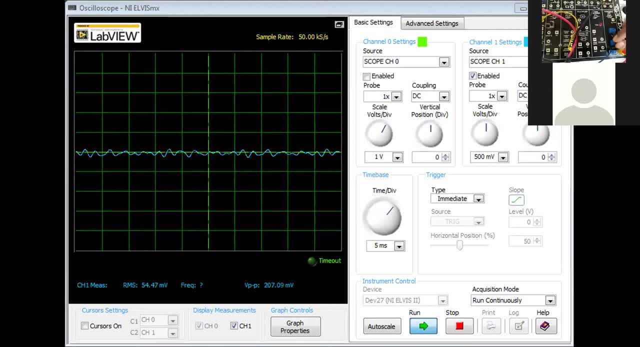 maximum, you will see the output. I'm changing the gain so you can see the output is decreasing. and if I change the gain to the or to the left, the right side, maximum side, you can easily see that. you can easily observe the waveform. okay, now, slowly, surely, slowly, slowly. 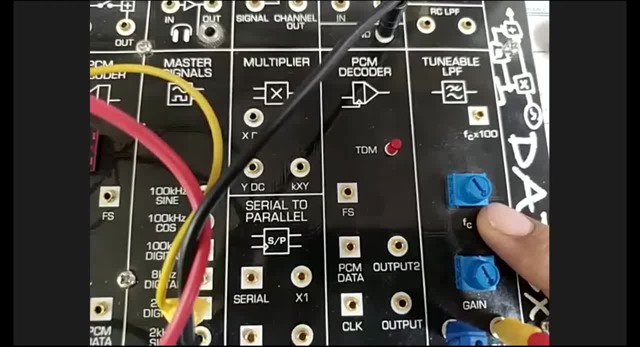 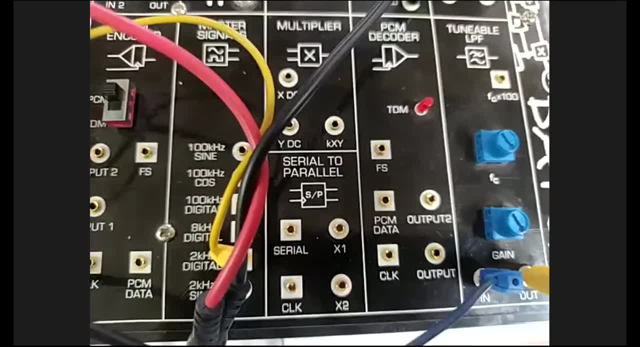 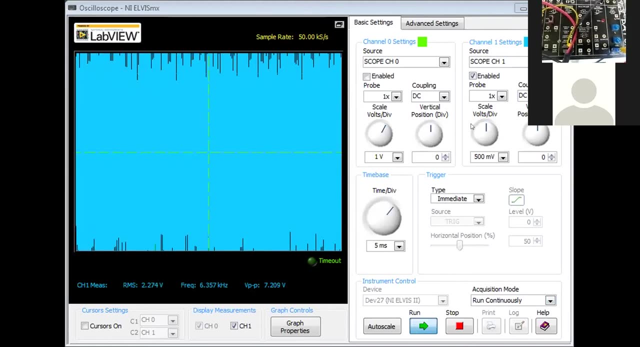 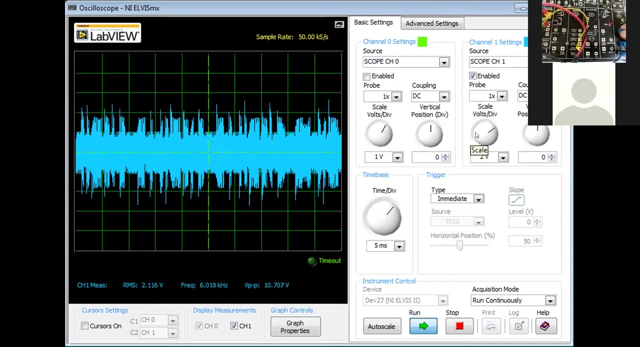 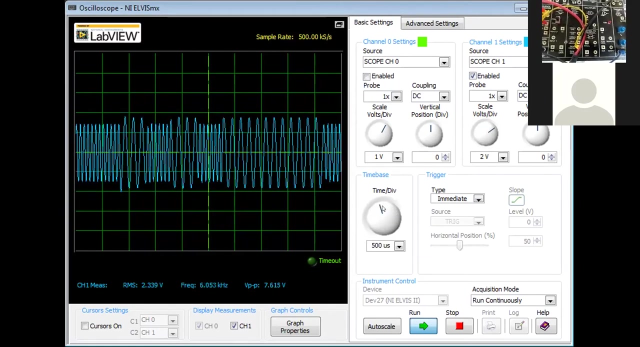 slowly tune this corner frequency. okay, I'm tuning this corner frequency very slowly to the left hand side. you can see the output. I've got the output over here. see, this is the mark frequency and the space frequency and I hope if I open this you can easily 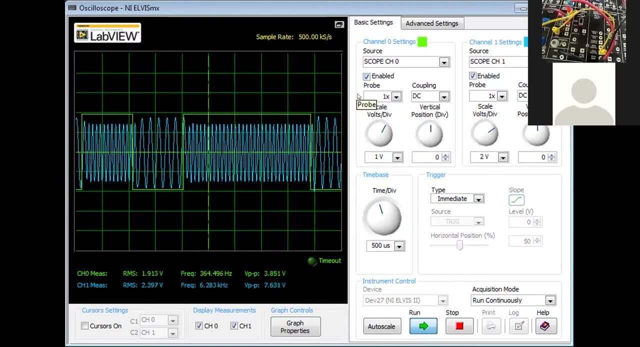 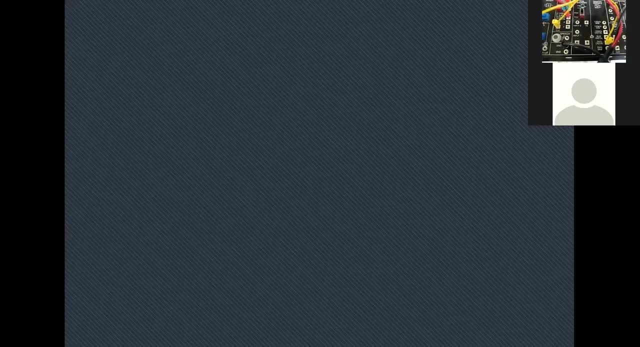 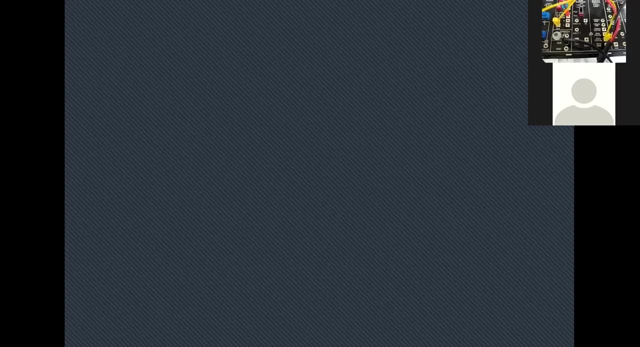 model the both the frequencies. you can easily see the both the frequencies. now we will move forward to part B and this part C. I will modify the setup and I will modify the setup such so that I'll you will see the output from the RC, the resistance and capacitance low pass filter on the channel one. 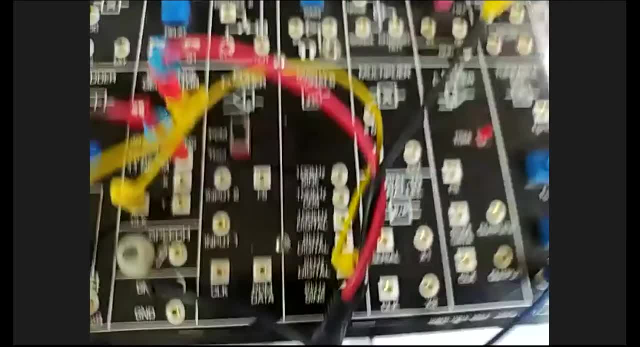 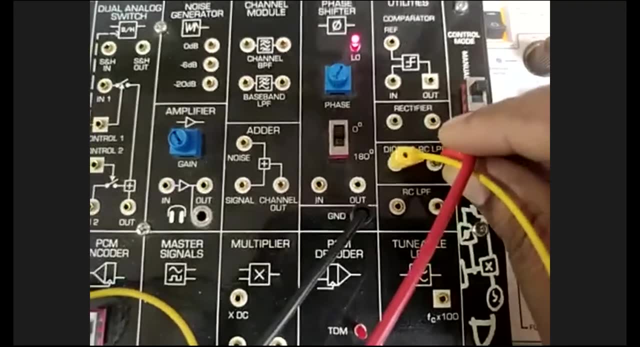 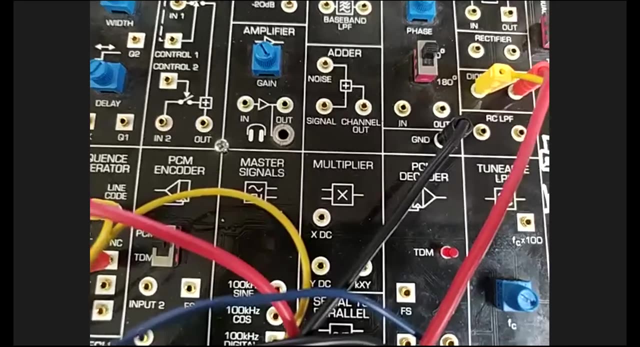 understood what I am, so now over here what I am doing. now I'm having- I'm moving the output to this or this position- RC LPF. now on the channel one I'm observing the RC LPF. so see, you can now if I change the gain. 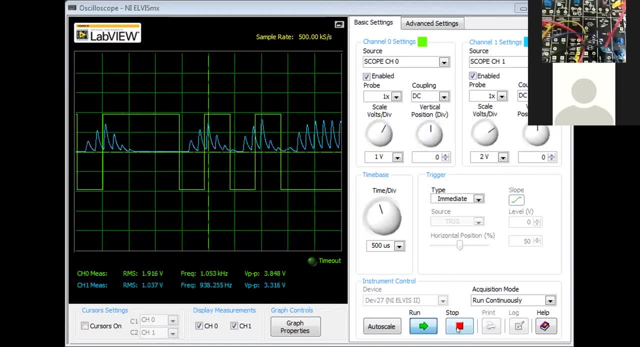 sorry corner frequency over here. I will stop this. you can see I have stopped this. you can see I have. you can see i'm moving. i'm slowly changing so that the mark frequency of the maximum frequencies are all zeros, approximately zero. this is a very tricky part of this experiment. 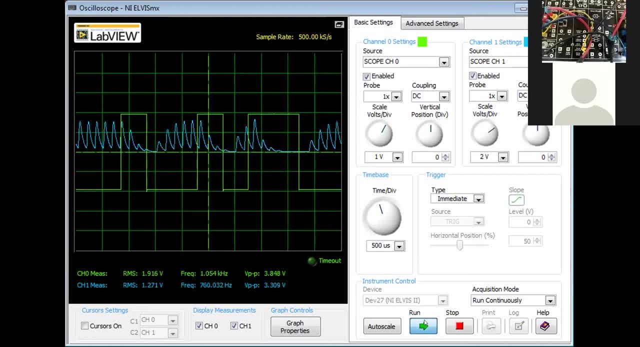 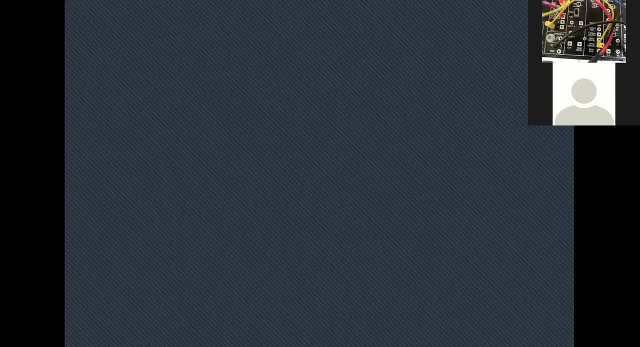 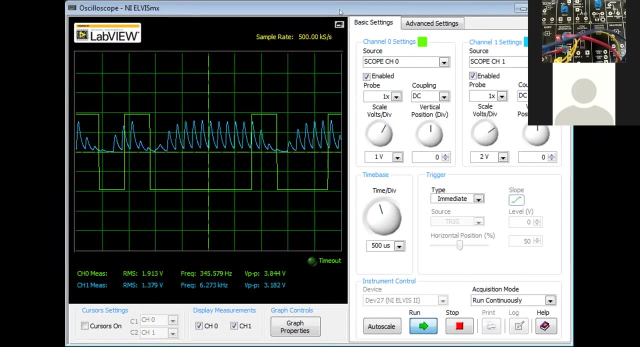 to model or to change the fc, because slight changes can occur in can result in huge changes. slight changes can result in huge changes. okay, the part c is basically restoring the recovered. part c is basically restoring the recovered data using comparator. now we have got the comparator over here and i will use the comparator signal again. modify the diagram. 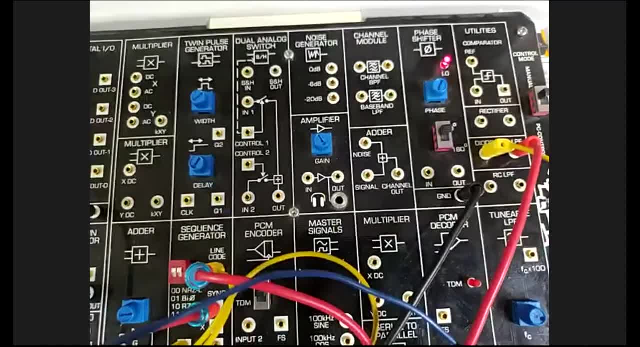 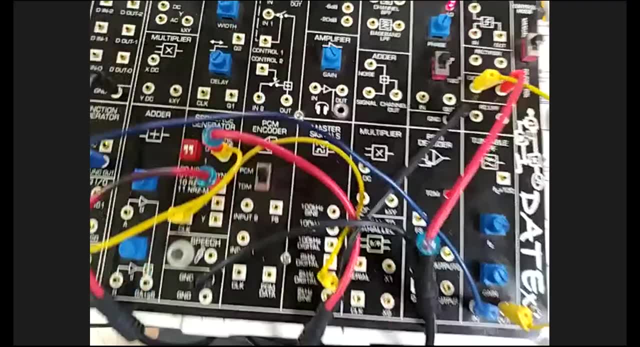 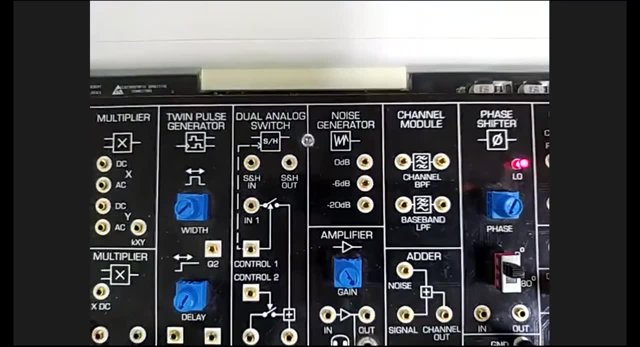 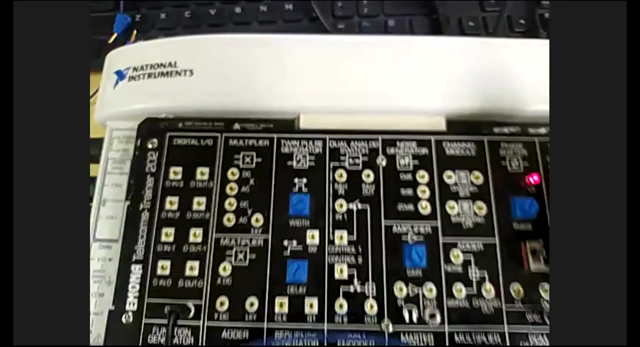 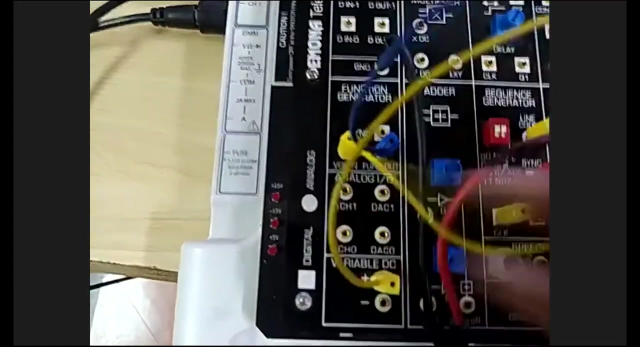 i will use the comparator, restoring the recovered data using a comparator and then all the comparator. i will use this variable dc supply positive side and i will use this comparator, okay, for the reference point. i will use the dc signal to reference. switch off the variable dc supply positive side. okay, and the 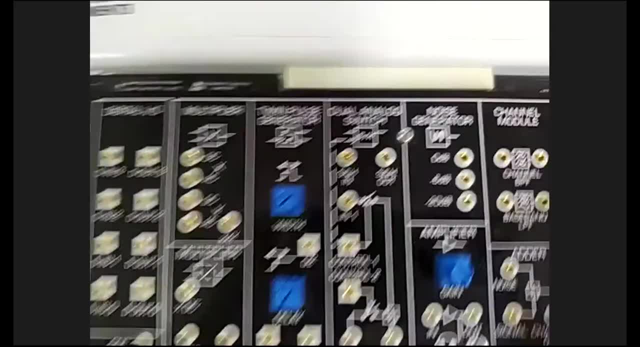 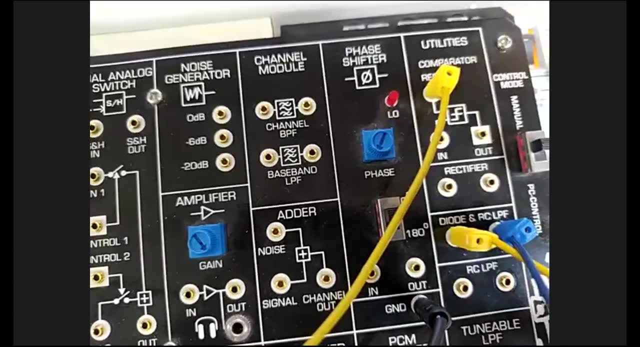 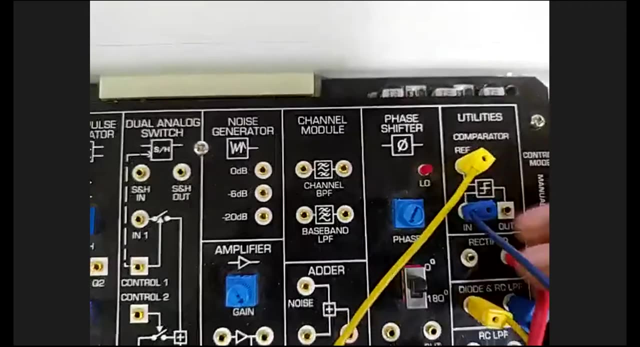 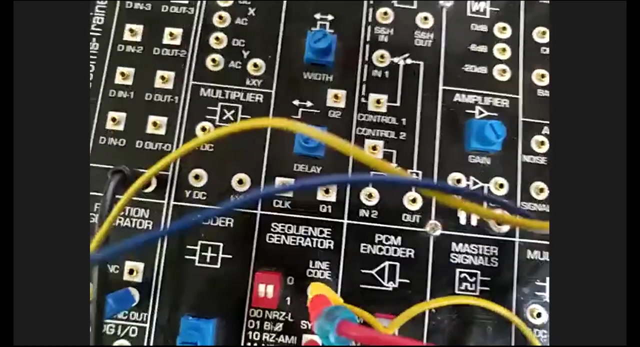 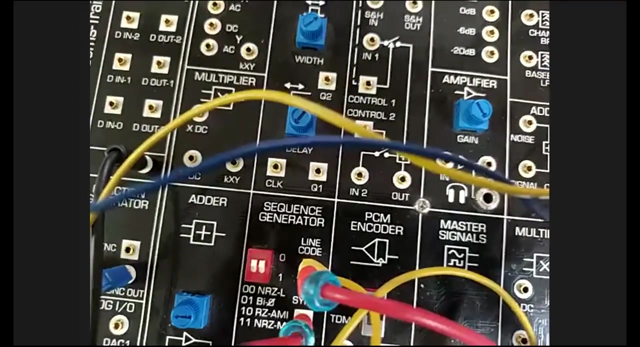 other part of the comparator's input is from this rpf. from this rpf take the input, another comparator, another input of the comparator and on the channel one or the output of the comparator. we will observe the output of the comparator on channel one. switch on for this. first we have to see, we have to set the variable power supply. 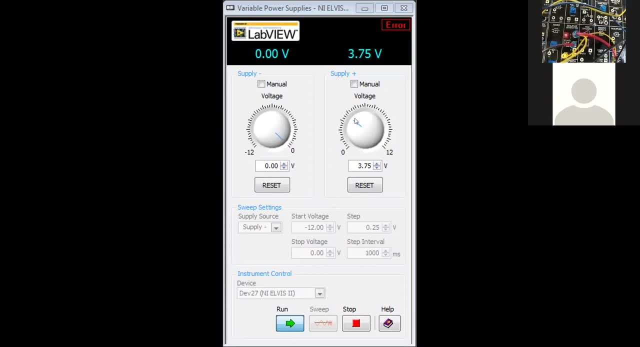 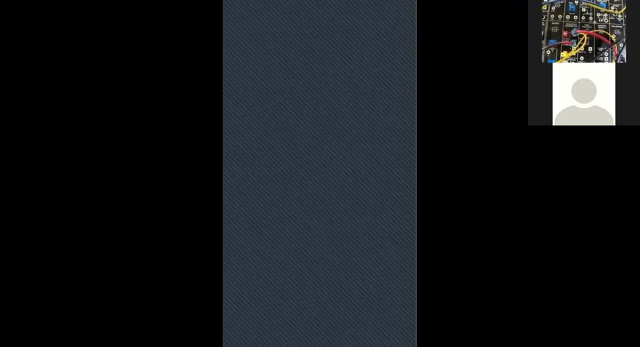 i'll use this variable power supply and i'll set this variable supply to to such that we can have the modulator signal. okay, now again turning back to the scope. i will turn back to the scope again. the system is on and i will show you, on the scope first, how the output is currently looking like. 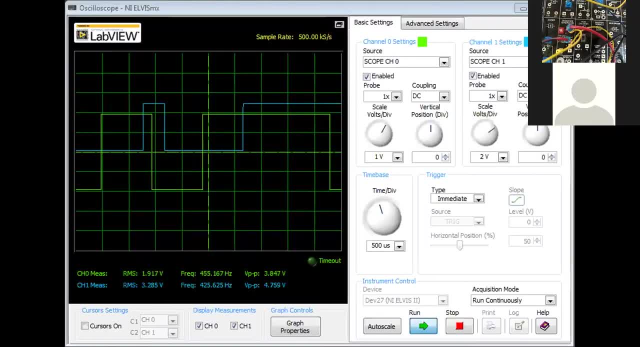 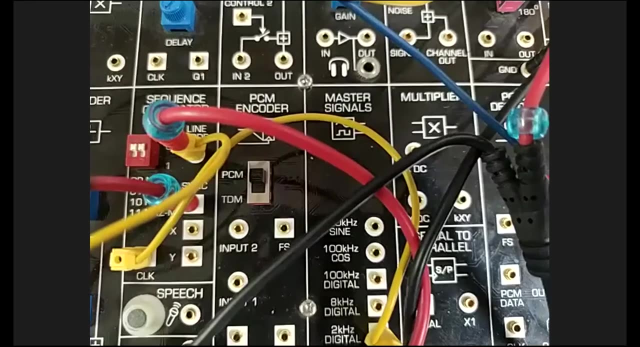 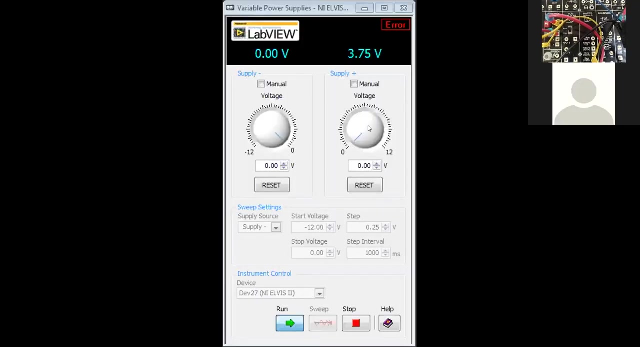 oscilloscope, oscilloscope, here we go, oscilloscope. this is how the output is being looking like. now i i will slowly turn the variable power supply model button. i'll show the variable. i will show you the variable power supply. okay, this is the variable power supply positive side. 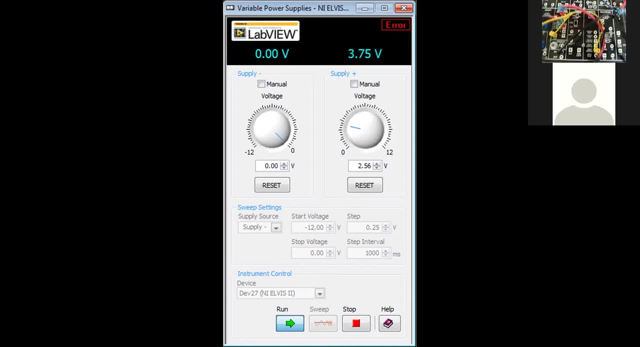 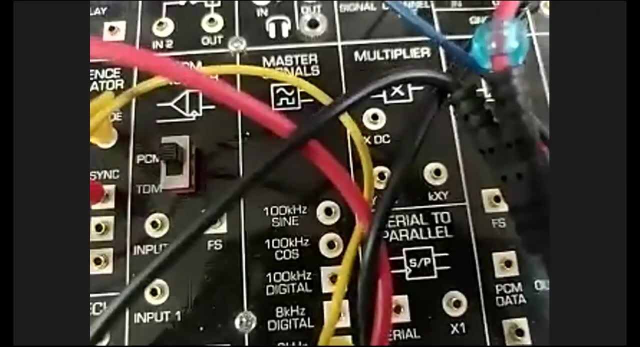 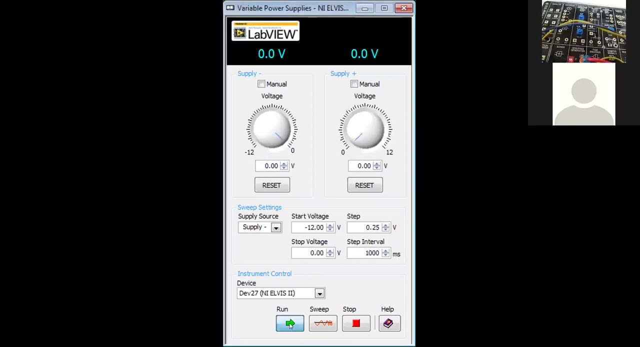 it is hanging right now, so i will show you the output. i will show you how the output is hanging right now in the scope. can switch frame rate in the scope. let me restart the variable power supply soft button because it's currently hanging. okay, this is the variable power supply, so i've i'll click on the. 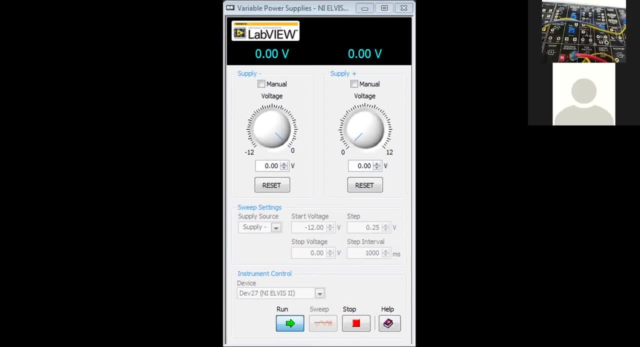 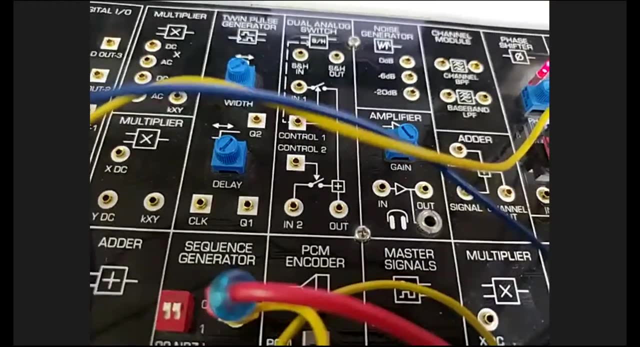 run button so you can see the output is changing. i will slowly change the output. you how the output of the oscilloscope is looking like and you will observe the output. i'll change the what you can say- variable power supply positive button. okay, over here you can easily. 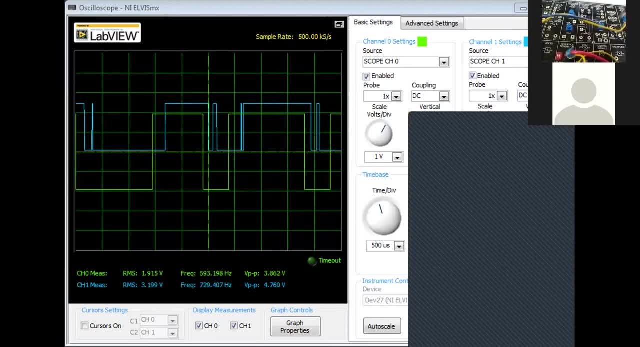 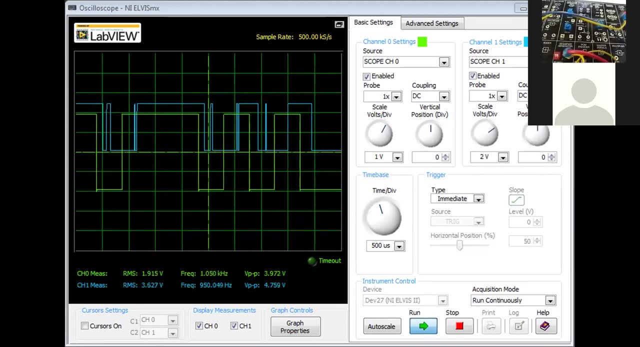 see the oscilloscope now. i'll see what you can say. let me move away now, i'll see. i'll move the variable power supply and you can see how we are getting some results now. okay, we are getting some results now. set the variable power supplies, positive output, to zero volt and then modify. 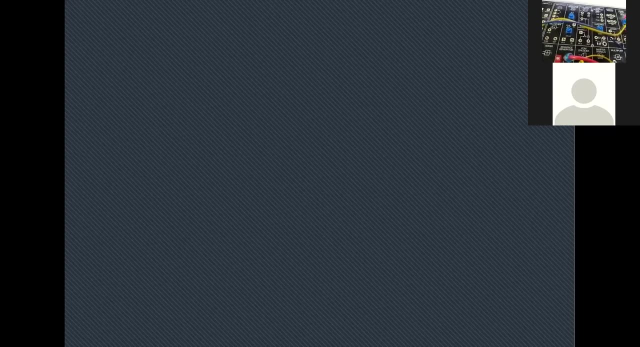 the setup. compare the signals. if they are not the same, adjust the variable power supplies- positive output, soft voltage control until they are. if they are visible, these require adjustment to the reference voltages close to zero. so let me show you the oscilloscope first. this is the oscilloscope.